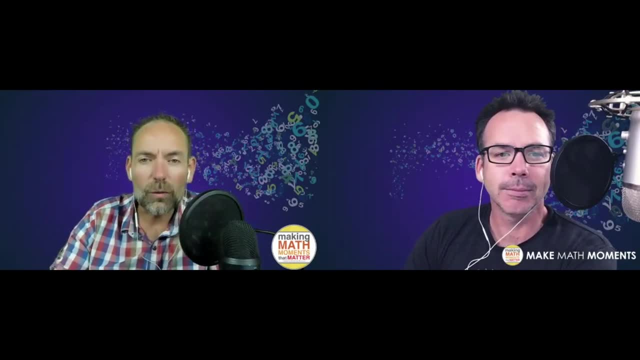 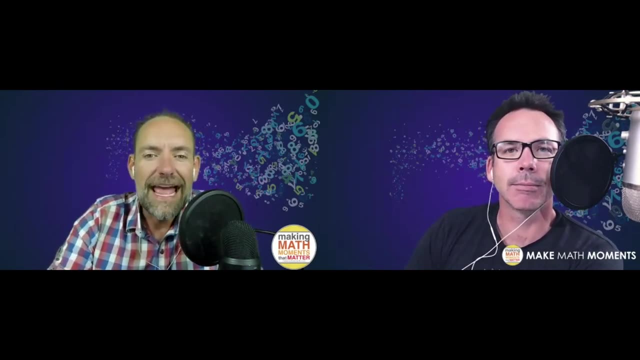 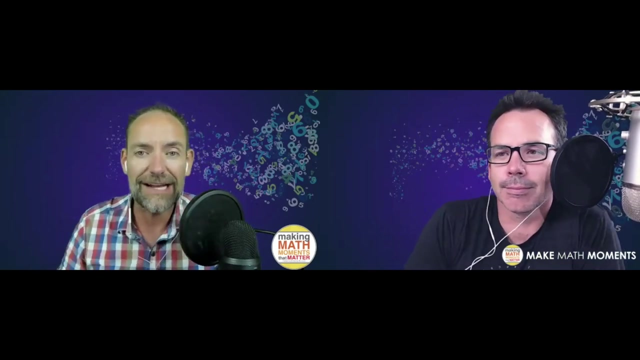 with you A community of math moment makers worldwide who want to build and deliver math lessons that spark curiosity, fuel sensemaking and ignite your teacher moves. Friends, we are so excited to come to you on your favorite podcasting platform, but also. 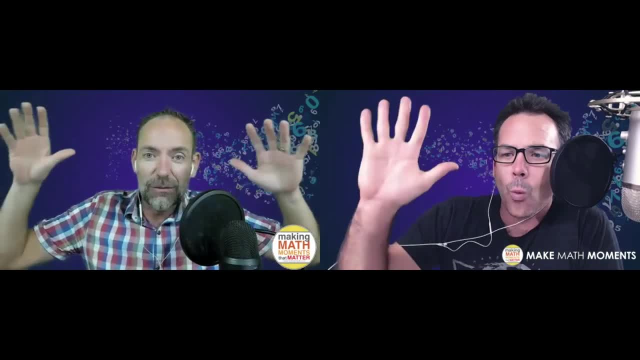 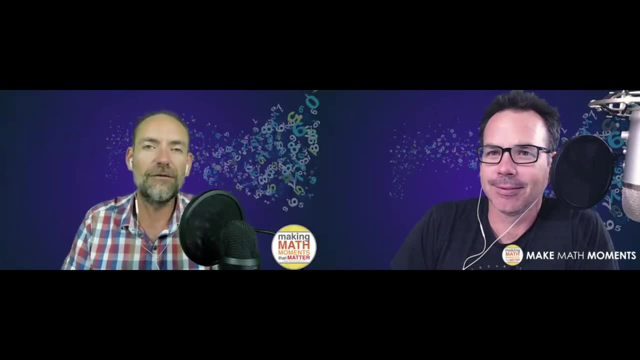 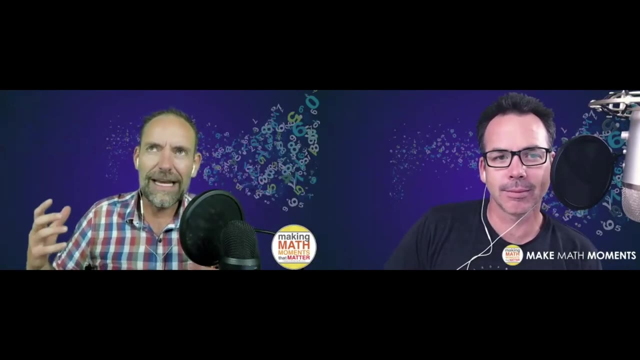 with video. You can see us if you're on YouTube, watching us on the YouTube channel. We are going to try our best to continue offering video opportunities for you, for the podcast And John, we've got a doozy of an episode here because I think it's going to really 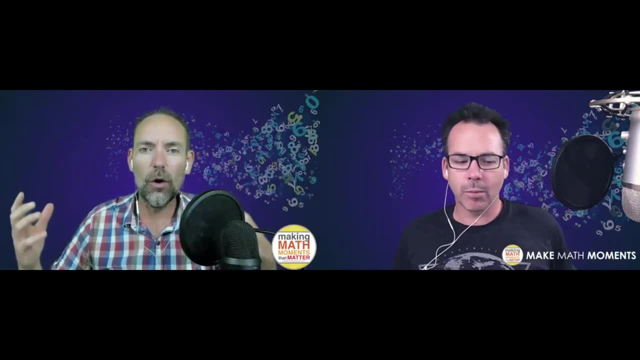 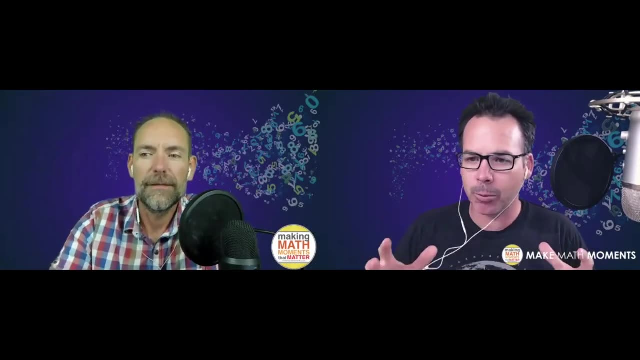 help kind of connect a lot of the ideas that we've been sharing over these 150 plus episodes of the podcast. Yeah, for sure, I'm really excited to chat with you, Kyle, about this topic on storytelling and how to craft a story, that and what are the elements that go into that kind of story. 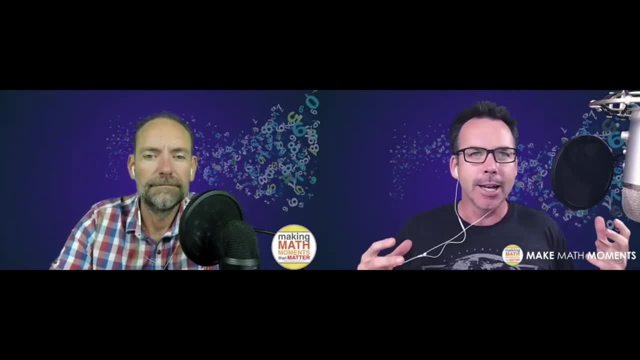 so that we can model our lessons around it. Yeah, absolutely Yeah. So we're going to kind of go around that and capitalize on you know this, this art form that's been around for forever that we've been using to communicate ideas and communicate. 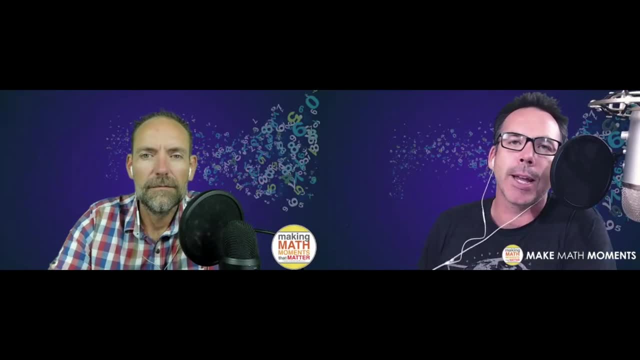 powerful ideas. Storytelling is that platform and- and we're going to do this here today with you- is is: how do we do this in the math class? And, like what Kyle said, it it kind of it kind of wraps around our mathematical you. 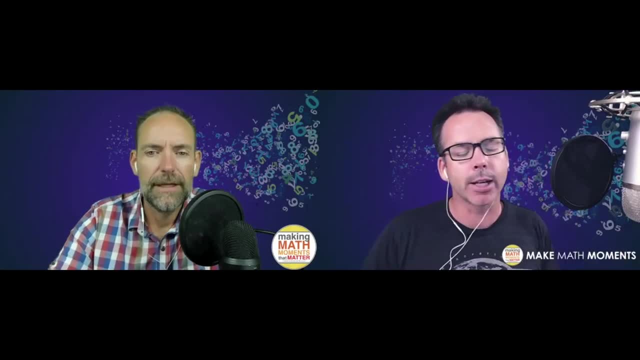 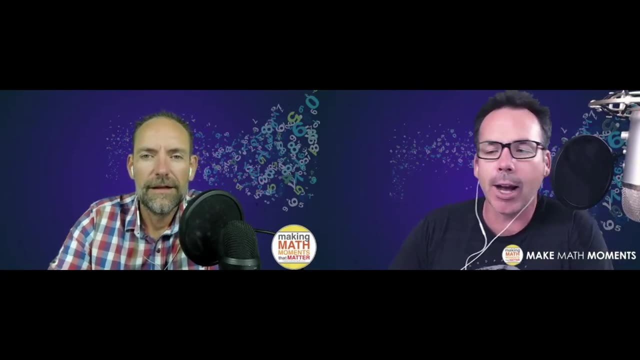 know our mathematics framework, that we've talked about our three part framework here for the Make Math Moment. Yeah, It's a podcast and also on our website, So looking forward to getting into that with you. Kyle, let's begin here in this episode. 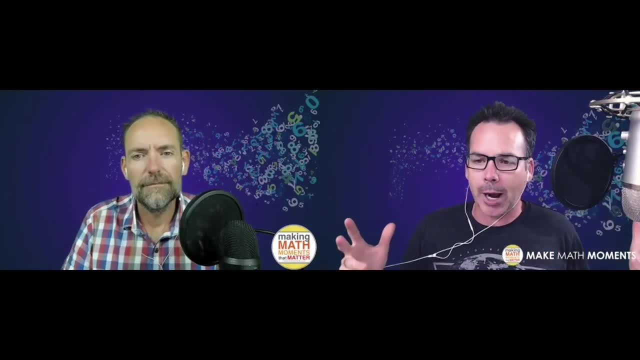 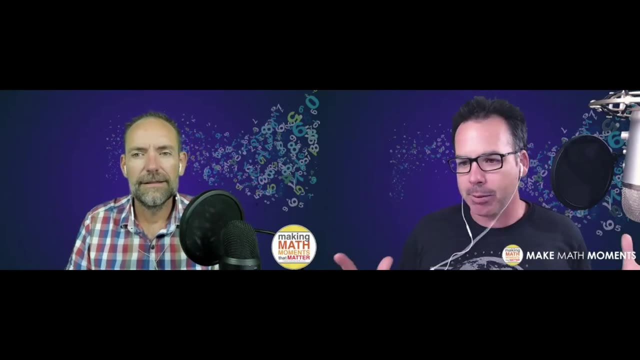 by telling you know, like, why, like maybe we should just like, why do we need to even like talk about a new model of of math lesson? Like like? I know that we've chatted many times about what our classes look like before. 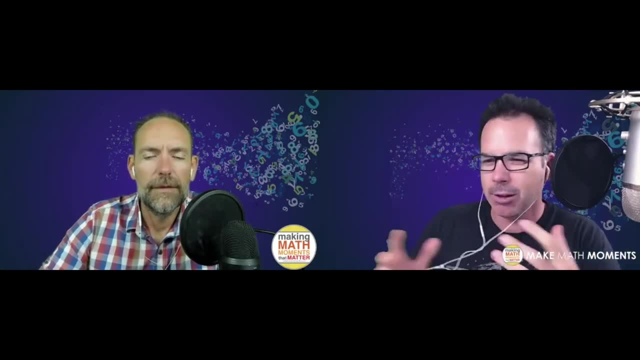 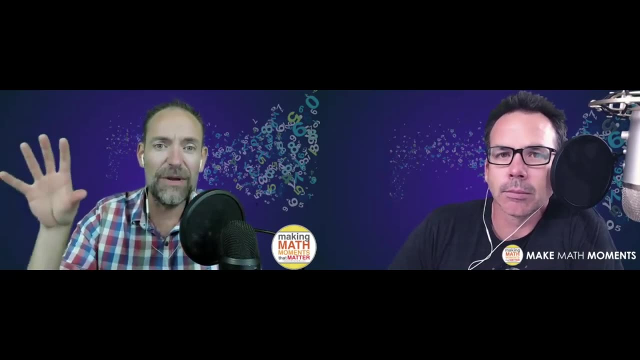 we've made switches, but let's let's dive into, like, why we need to make some changes. Yeah, Well, it's actually interesting because you were talking about storytelling And we we think about story as something that has been around forever, right? 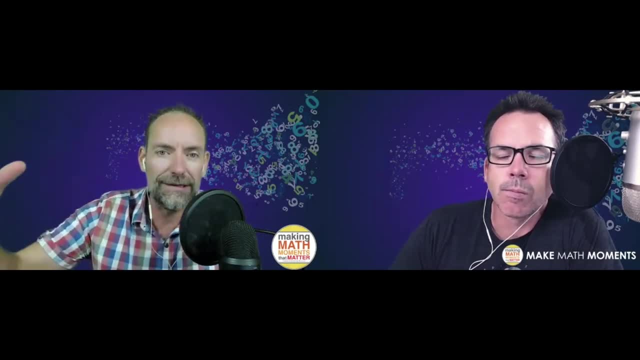 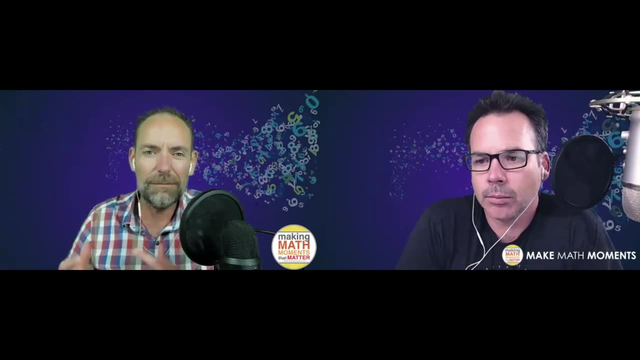 And some of the best legends, some of the best stories, some some of the best history is told through story and those tend to stick right, Like when somebody tells you a story, especially when there's like a lesson to be learned. you. 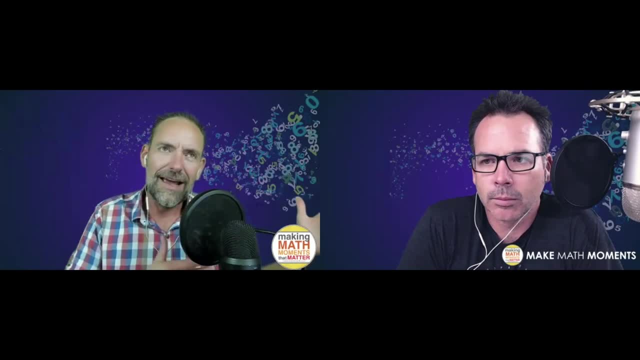 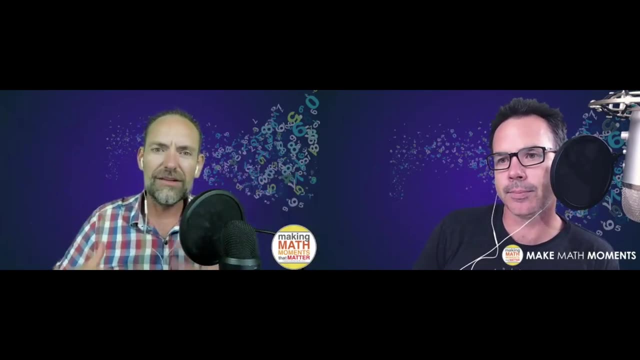 know they tell it through story, but yet when we look at math class and we think back to at least again, the experience that you and I share quite often Is that it wasn't really a story. It was almost as if we had signed up for math class and really wanted to learn and just 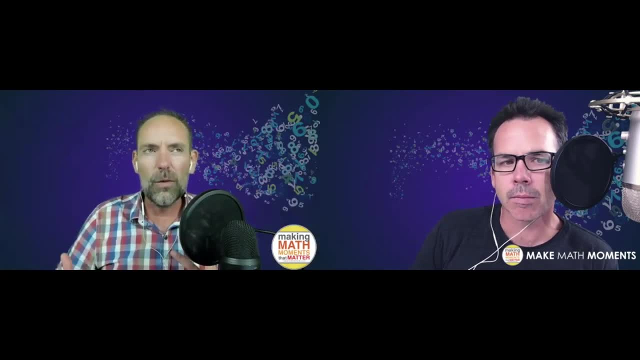 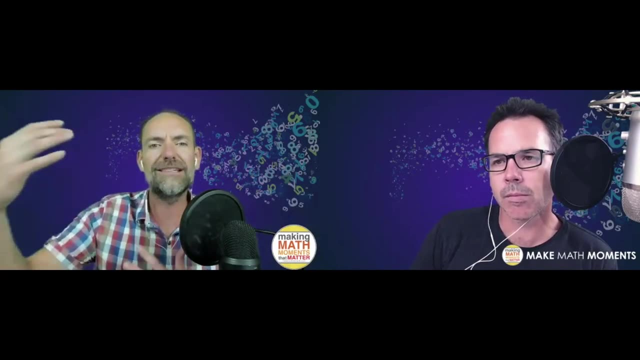 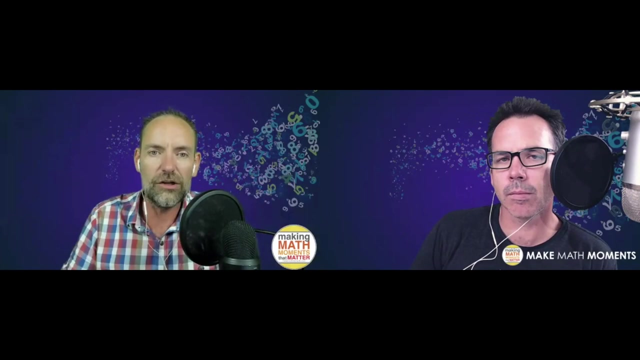 sort of expedite the process, When in reality we were just sort of sitting there as students that had to take this information in. I just wonder how much more of it would have stuck Had we had experienced that storytelling, you know scenario or situation. 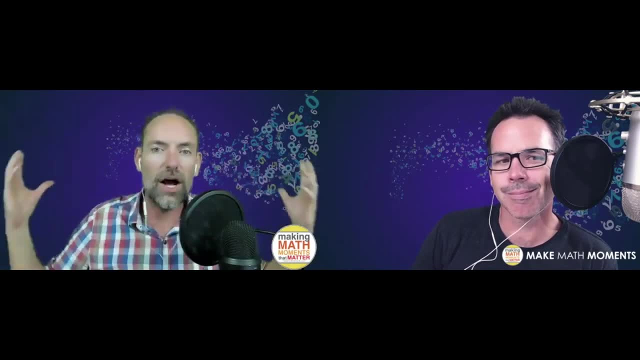 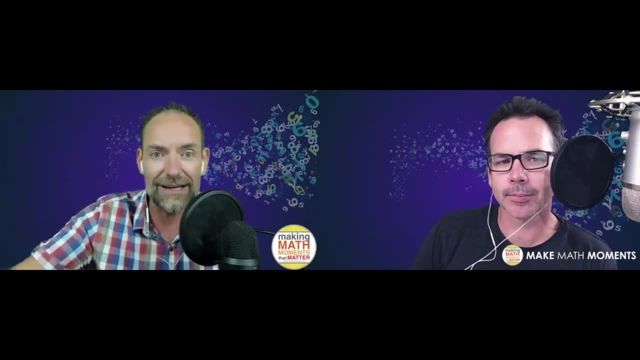 a lesson, And why did they tell it through story instead of just telling the lesson: right, Right, Don't, don't fly too close to the sun, Like that's all you need to say. Move it along, No, they told. 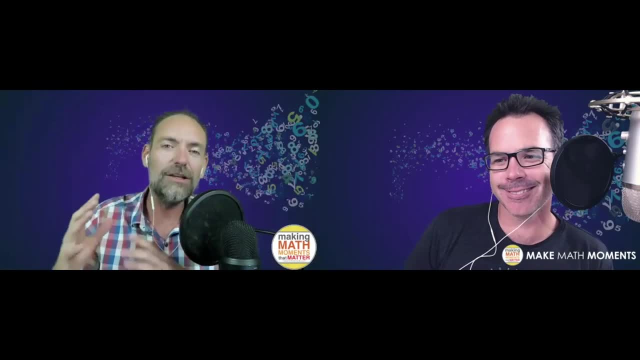 Copy it down in your notes. Copy it down in your notes. They told a huge story around it so that it would resonate, so that it would stick, so that you'd remember it And then, hopefully, you'd be able to put it into action. 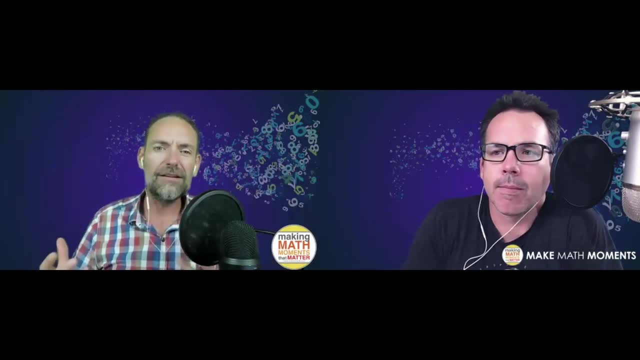 And John, when I think back to that gradual release of responsibility model that you and I both kind of remember as students and also used as teachers for quite a long time. I know that sometimes we try to throw in some maybe hooks or storytelling elements, but they certainly don't. 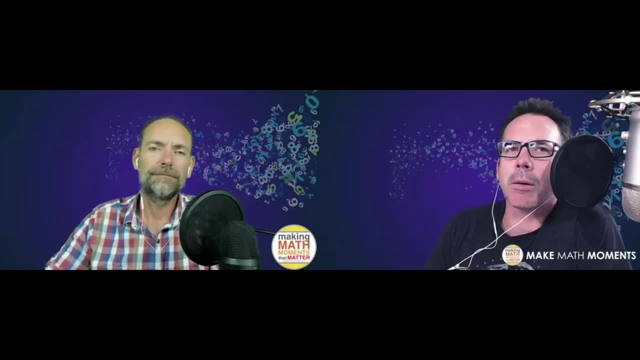 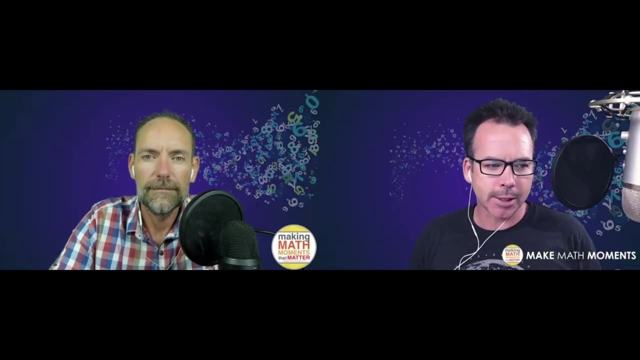 seem to play out like a story. Yeah, And when you say hook, I just think back to my days as a student teacher and you know, sitting in pre-service classes and they're saying like you gotta have a hook to your lesson, And what they're trying to, what they were trying to say back then, is 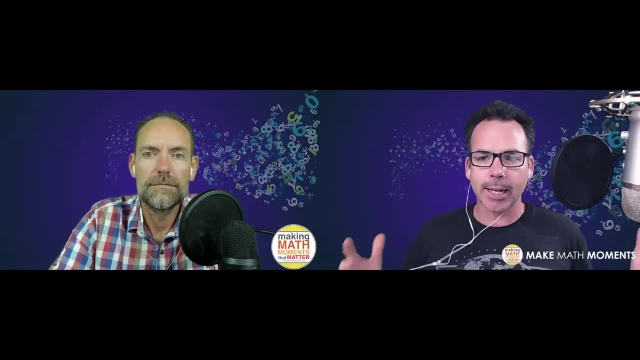 how do you think you've got to craft your lesson like a story so that kids can be hooked into that, that, that, that, that lesson, that idea, what is the big idea you want to? you want to bring bring about And, and and I, and I think that gradual release of responsibility, like the way 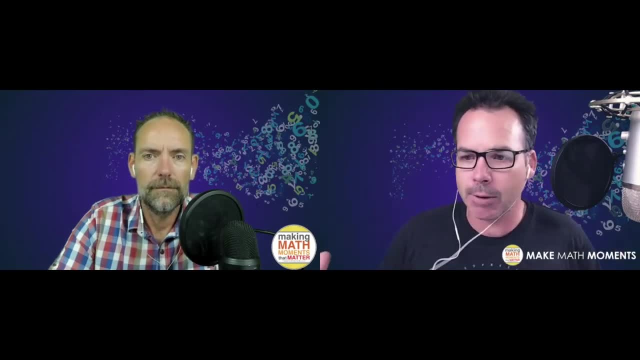 that I was designing my math lessons was. I was. I wasn't even like. at times I was like: let me, what is the hook? But the hook was like: I'm going to present this math problem that it's hard, that we may not know how to solve, And then we're going to show you how to solve it. 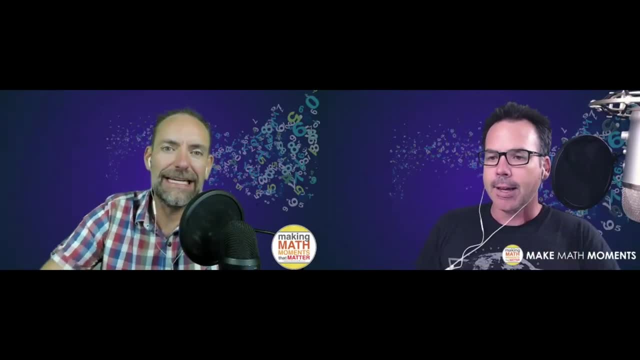 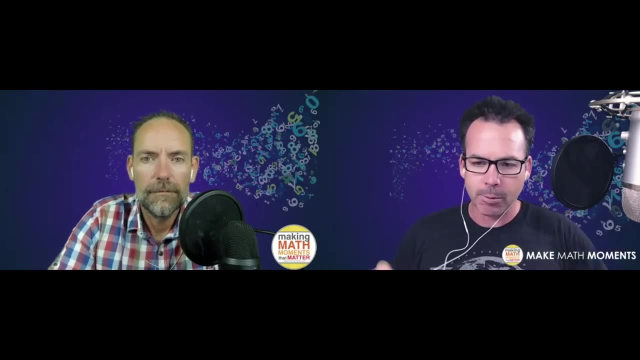 And I'm going to make it easier for you, right? Like somehow I'll make it easy, Yeah, And just it was. it was today, we're going to learn about this, And I would write the goal on the blackboard. And then it was like: let me show you how to do that so that you don't struggle. 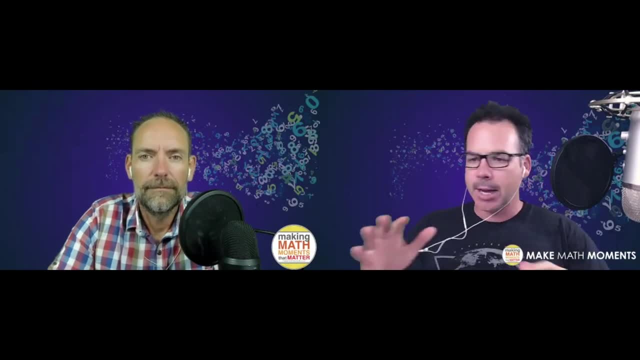 at all. Right, Like you're not going to have any, any sort of worries, You don't have to think about. you know what, what to apply. I'm going to show you the steps that are needed so that you know you can get through this, And I- and I think why we did that, Kyle. 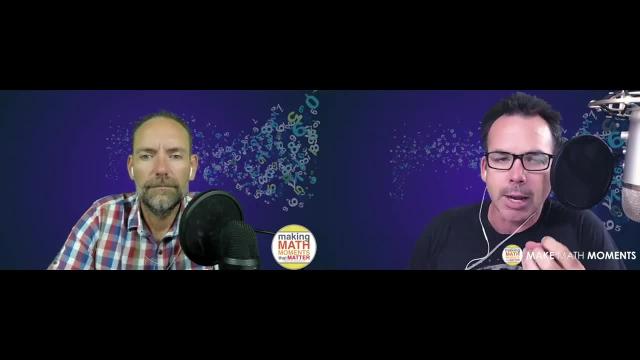 is because we knew. we knew that, that most of our students struggled with math class, right Like struggle with math. They hated math. Even even the kids who didn't hate math. they would be like I find this part tough, but not this part, And it was. it was we're coming. we were coming from a 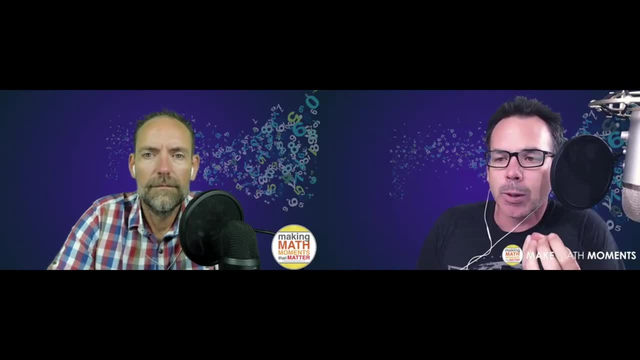 place of help. I wanted to make it super, super easy for students to follow. I thought that was being a great math teacher is if I could, if I could make this as easy for you to follow, you would be, you would be fine. And what I was, I think, forgetting, or what I learned later, 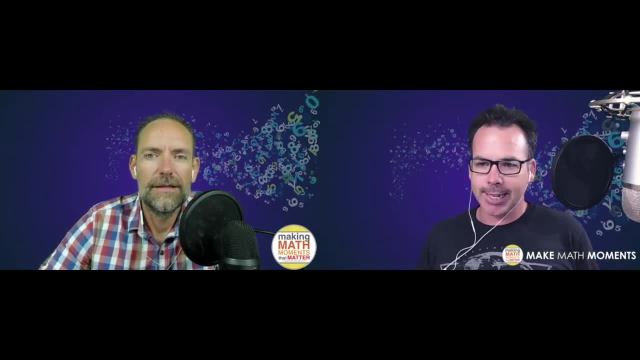 was that? I think it was, it was the struggle, It was. it was this like toughness, that this this problem solving aspect that I was leaving out and just telling kids how to solve problems instead of letting them experience that, And I think I think we missed out on a lot there. 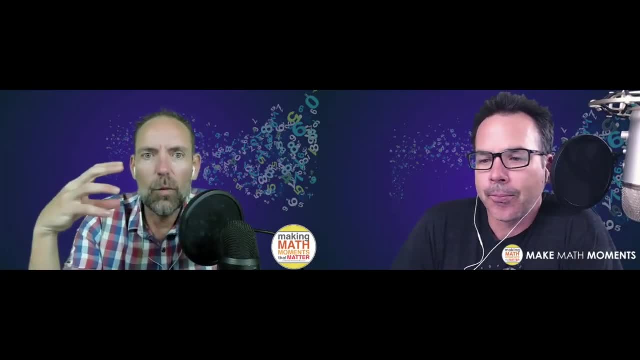 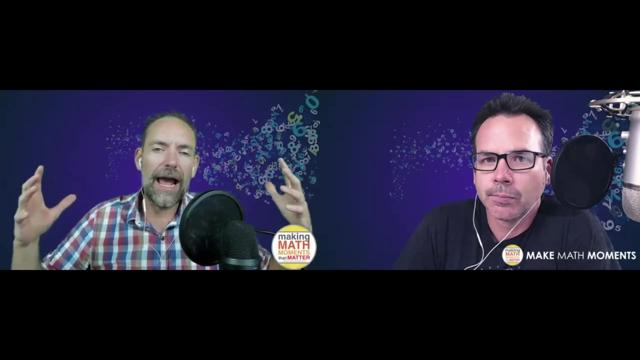 When you, when you go back to and you think about stories and the reason why a story is what it is is so that it's like the lesson sticks, And when we think about how you and I were both and we can't speak for everyone else listening. 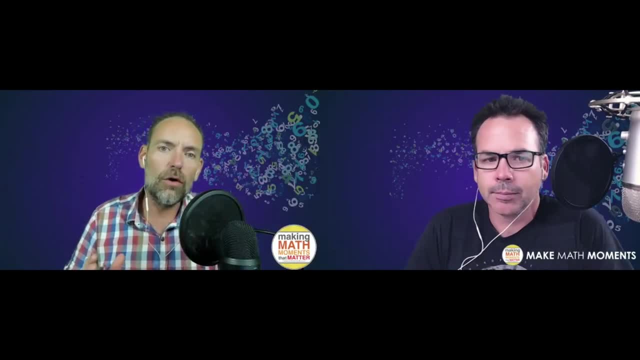 but how you and I were designing our lessons. it was like we just want to get you over these little hurdles, Like every day was just a hurdle. Once you're over the hurdle, what was there to sort of like remember what was there to kind of like you know, connect my thinking in my 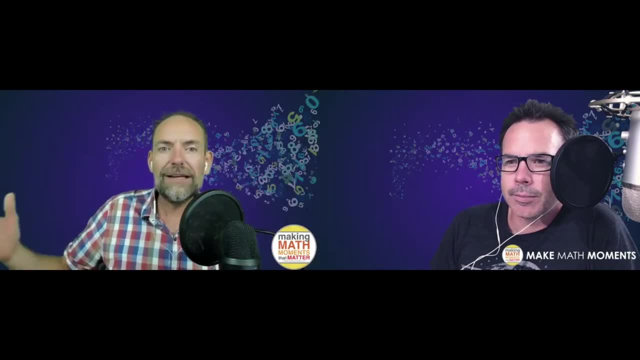 you know the work that we did that day. And then we would go like weeks later, or sometimes months later, when we go to the end of a semester, a standardized test or an exam, And then we'd wonder, students, it was like we had to reteach everything And it was like nothing ever stuck. 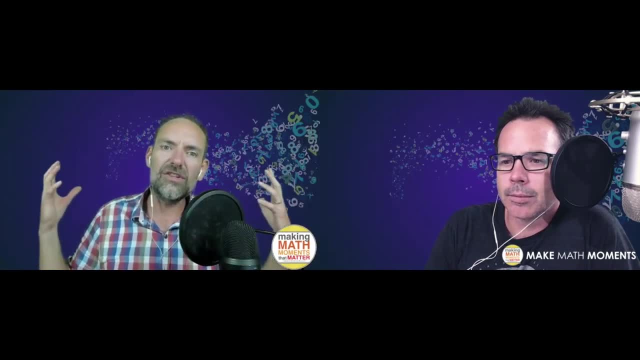 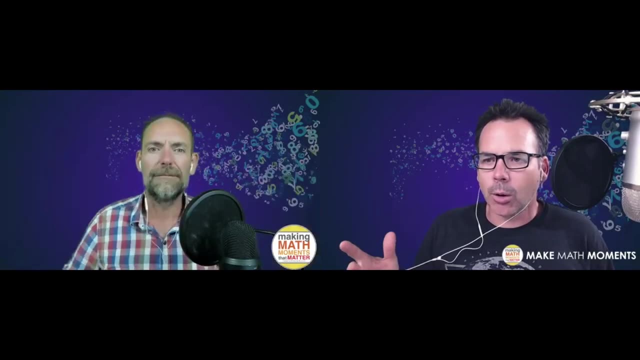 Well then we sort of start thinking and go, but there wasn't really like a story to remember there, right, It was just all these little disconnected pieces floating around that didn't really have a meaning Totally, And I think we were just, we were just hoping kids, 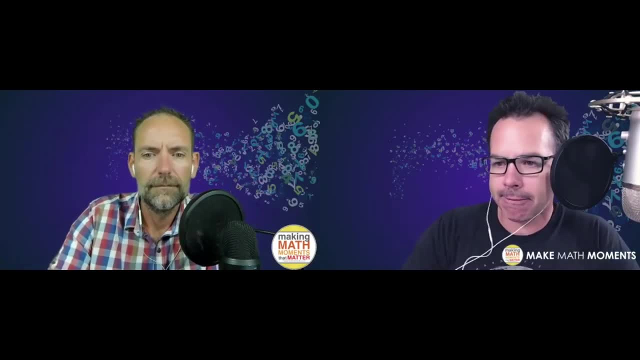 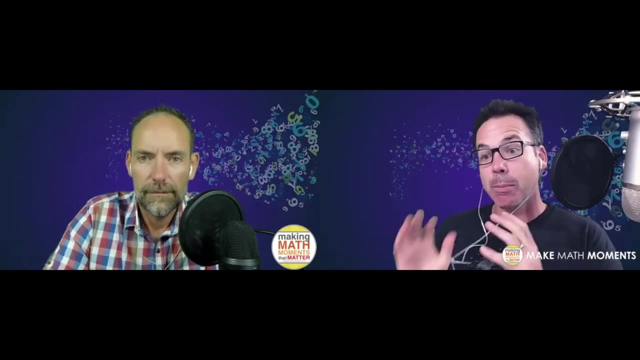 would memorize the procedures or if, like, we do it enough, that will become second nature, right, Like, like a lot of times you would relate it to basketball practice. You're like you got to shoot so many times so that you can. just your muscle memorizes And we'd say, oh, math is like that. 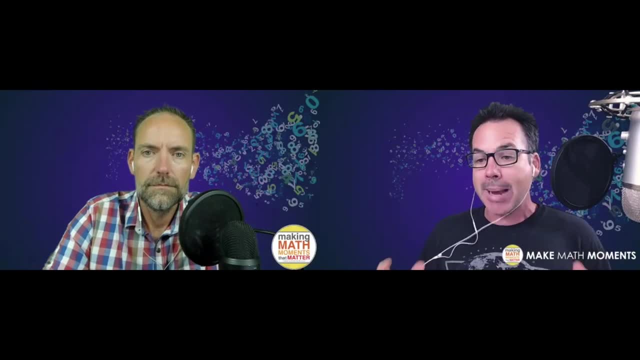 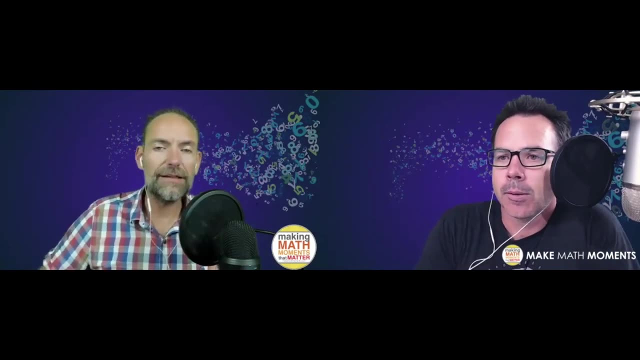 But I don't think math is like that anymore, Kyle. I think math is more about making connections instead of just repeated action, Absolutely, And you know. and of course we want purposeful practice, we want all of those things, but it's like based on what you know, so where's the 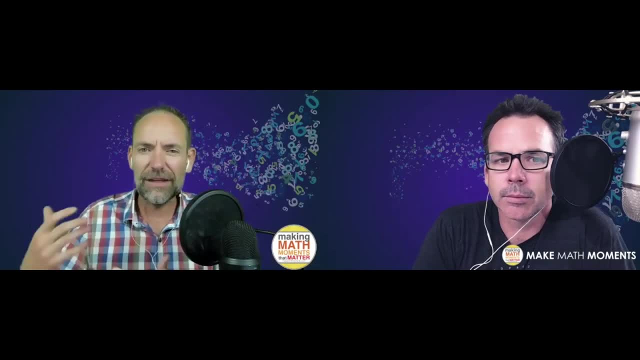 story, And if there is no story there, then you're just kind of repeating something over and over again And hopefully it'll just automatically happen, right? So let's talk a little bit about of storytelling, And I know inside our online workshop we have a lesson on what we call the 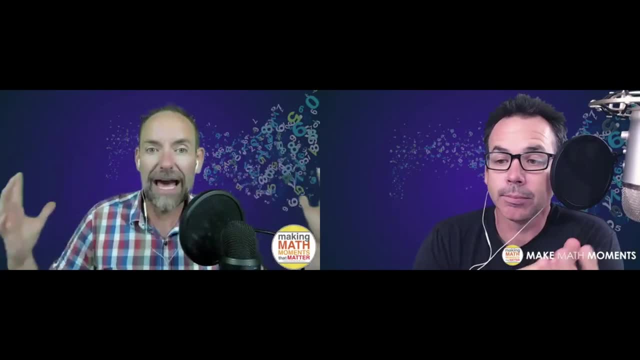 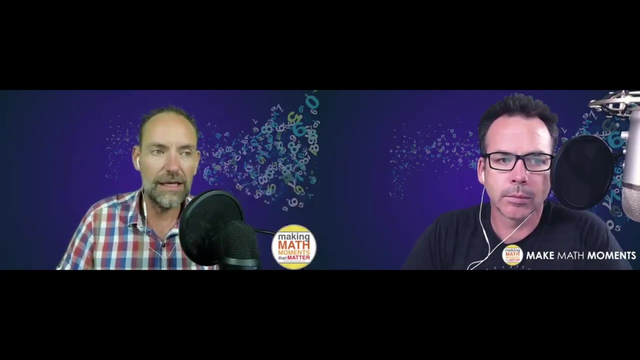 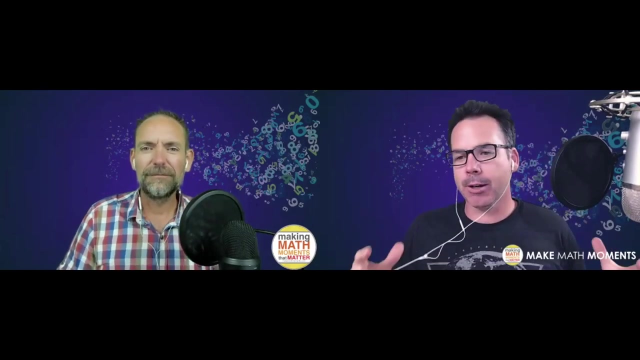 hero's journey. I mean, we don't really call it that, we just apply it to math class, because this is actually something that was shared with us at a workshop we were at. you know, one of the- I'm sure you remember Joseph Campbell- was. Joseph Campbell is the author of the of the heroes. 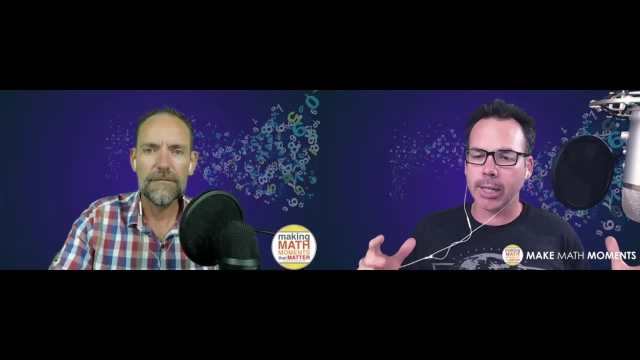 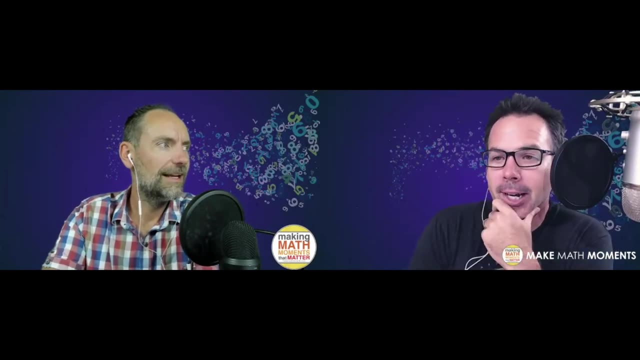 This is the person who wrote about the hero's journey, And he wrote about the hero's journey as a cycle, as a model of storytelling. We learned it. I know that you were where you're going with that, Kyle, as we were at- we were at an Apple conference, a 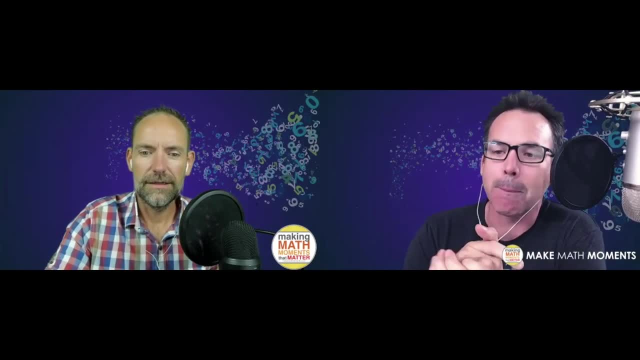 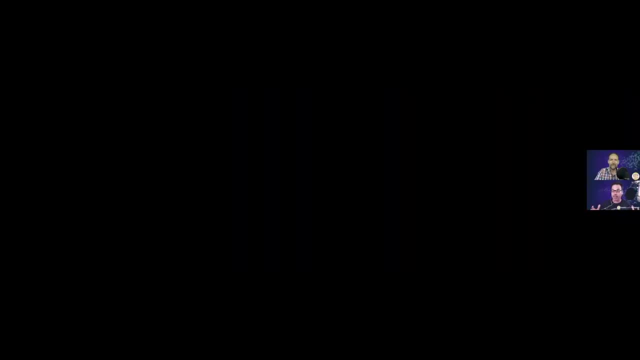 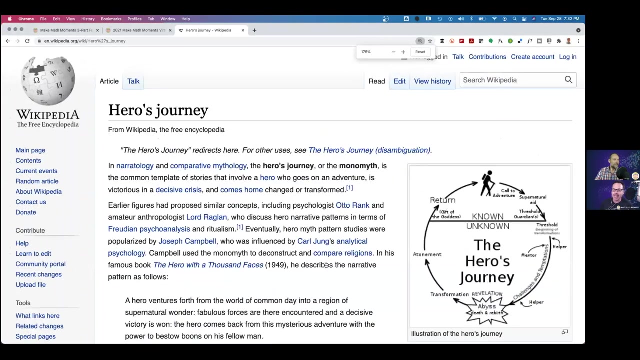 number of years ago and the head of storytelling from Pixar Studios was there, And you know what I'm like you. I forget the gentleman's name, but he was an amazing storyteller. This is probably why we remember this part of that conference is: is that he brought up? 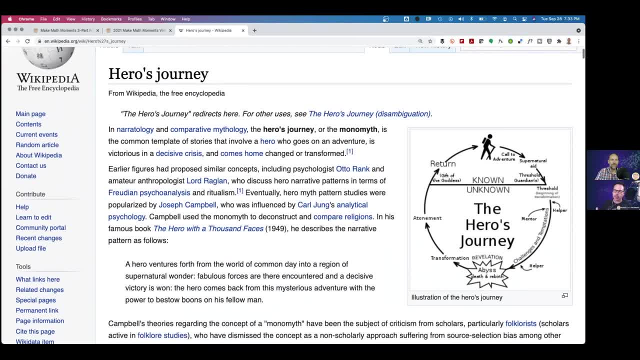 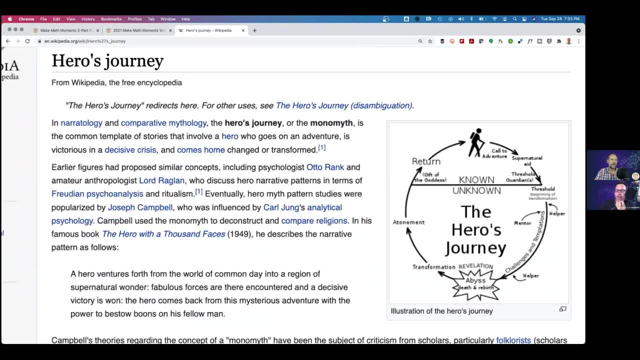 this, you know this hero's journey as this act of storytelling and and it really stuck with us And you know, we're just gonna, we're gonna, I want to, I want to outline this for for our listeners here, because because on the on, on YouTube, right here, we have some visuals that 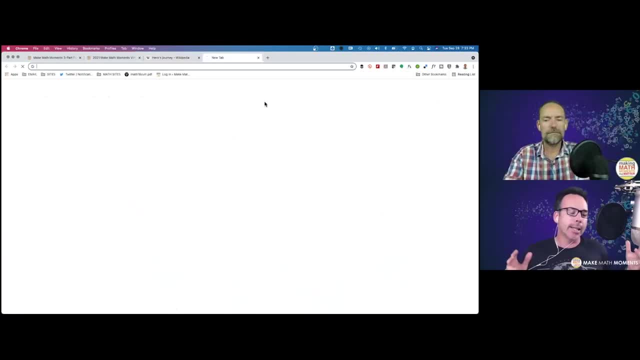 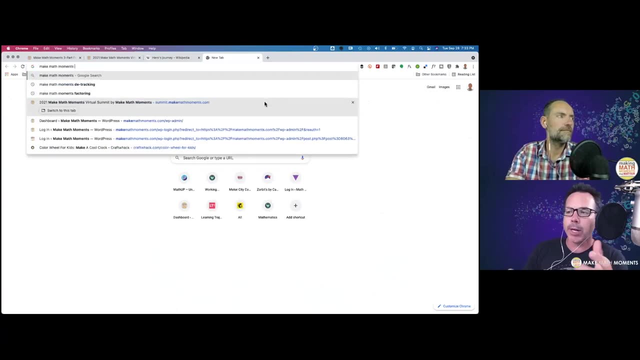 are coming up, but we're going to describe them here for you, listening at home or in your car, wherever you're listening to us right now. But the let me describe the hero's journey And what we do. what we have done is we've put this: 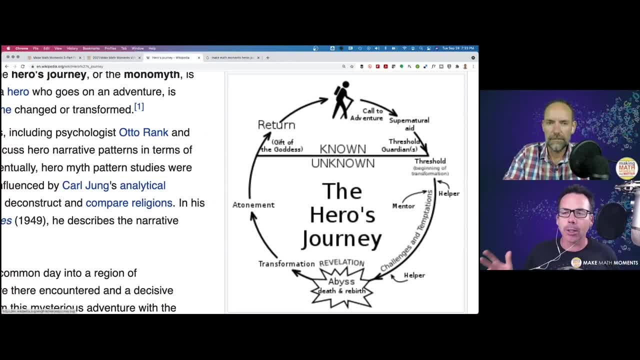 as as a like a graph. you know, like this is: if you Google hero's journey you're going to see like a cycle because of the way this journey kind of carries out. But basically the hero's journey is a model of story that every single you know, popular story that you know about that you're. 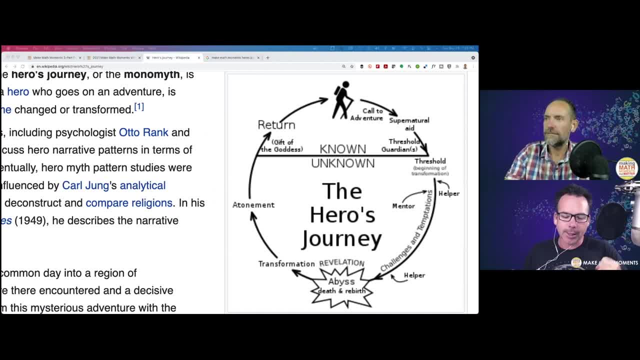 like I loved that adventure story. I love that you know science fiction story. I love that love story. like they all have the exact same story arc And that's what Joseph Campbell talks about in the hero's journey: it's, it's, it's this exact. 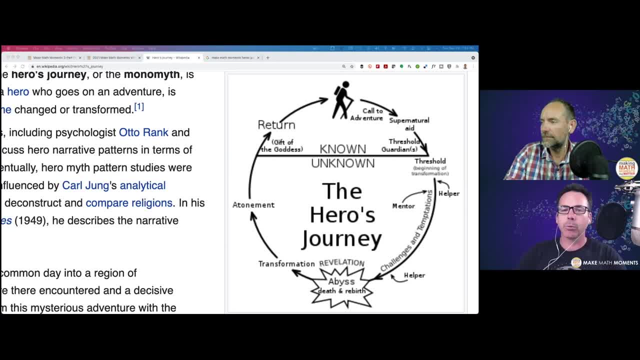 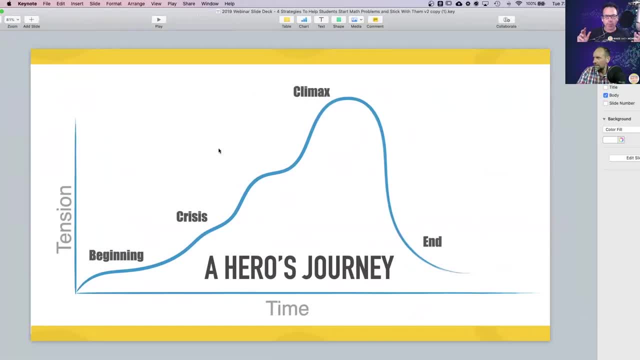 same story arc and I'll just gonna describe it to you. And what we've done is we've put it up on a graph and I'm going to share that up on my screen here, Kyle. So, so what, the hero's journey is. 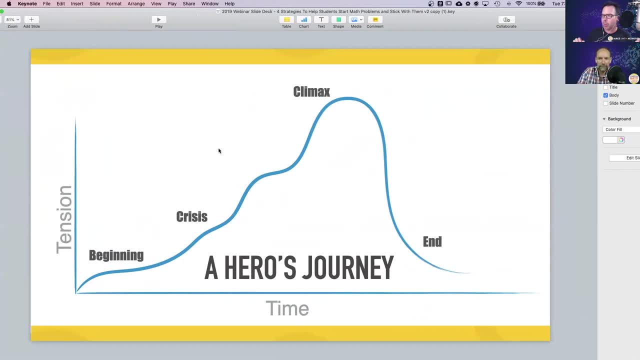 and if we put it on a graph? this is what we math teachers love to do, right? We put things on on graphs that we can understand them better. I want you to think of the horizontal axis as the time, like time of this story time of this, this game. you know, when you're right back at the top, you're. 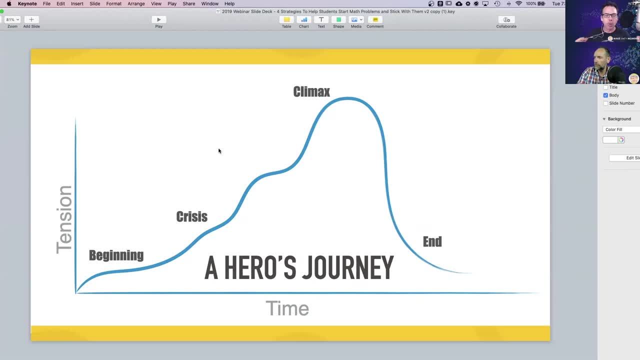 this character on this path in a movie, in a book, in a TV show, And the vertical axis is the tension. This is the tension that the audience will feel watching or reading or participating in this story And every single story. Now I'm going to use my favorite one: Kyle. 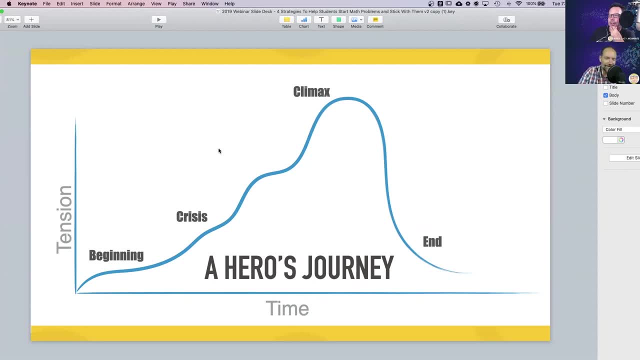 Do you remember what my favorite reference here is this? for It's definitely not my favorite, I know I will say that, But I'm going to let you have your fun. Have your Star Wars fun, Yes, Okay, So we're going to relate this to Star Wars. 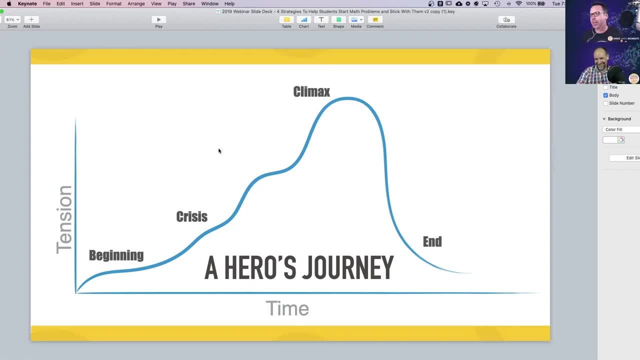 Kyle hasn't seen Star Wars, I think, So don't hold it against him And have absolutely no plans to watch it. This one perfectly fits this hero's journey, Because lots will fit this storyline. So every story starts the same way. 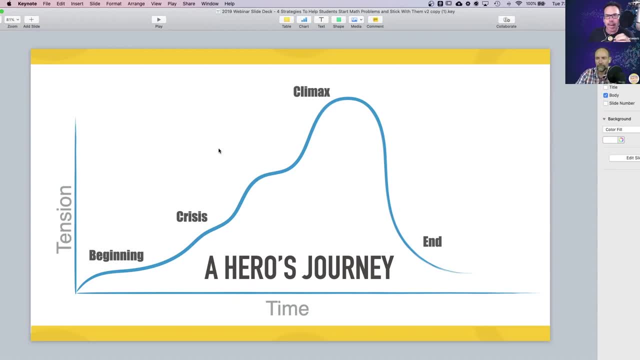 In the beginning, the character is always set in their world. They are in the world, In their element, And then, when something changes and they're set on the path, They're set on this journey, They're set on this mission or adventure. 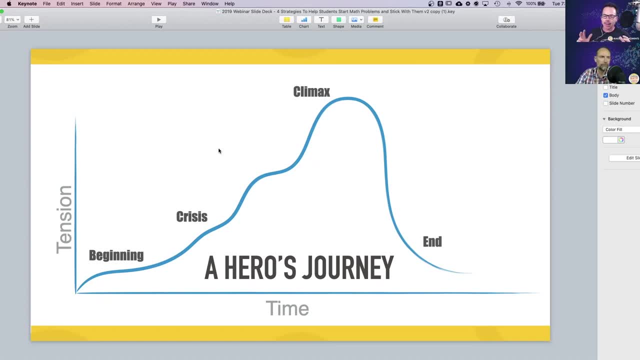 And what happens is the tension starts to rise And they're kind of going along this path, And what every hero must do is they have to. in that journey, they have to battle the forces of evil, They have to overcome struggles that teach them things about themselves. 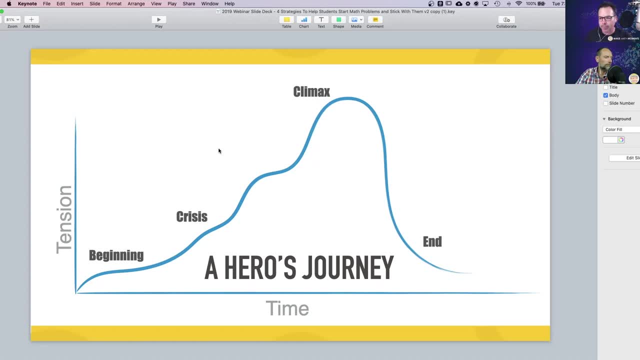 teaches them about the people that they're with. It's this crisis that the hero will go through. Every story has that part And usually along that crisis the hero will meet a guide. So if we pause here for a moment, Kyle, and think about Star Wars, 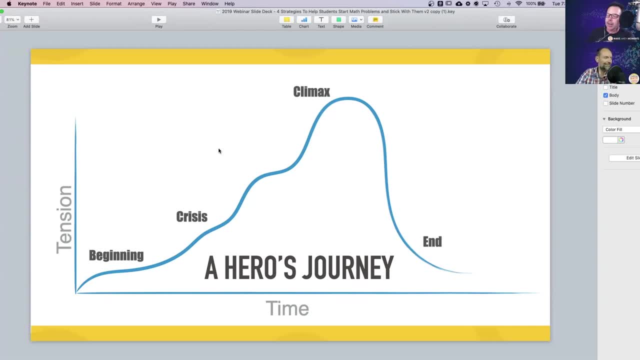 For all of these listeners who have seen Star Wars, except for you: Luke in his own world. right, He's in his world. He's a farmer. And then, Luke, Some terrible tragedy happens And he decides he has to leave his world to travel and go through these battles. 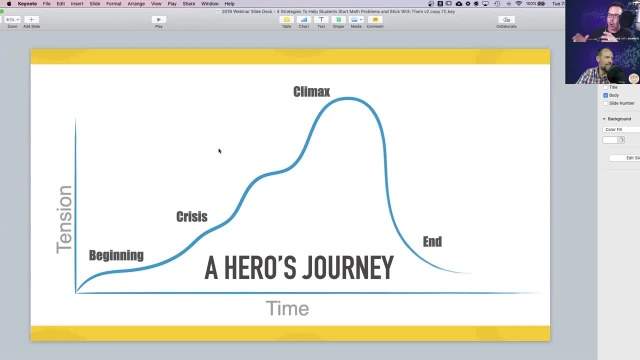 He has to go through this struggle, But along that path he meets Obi-Wan Kenobi, who's his guide through this struggle part. So every hero has that guide. Now, when we saw this at Pixar, remember the story that this gentleman shared with us was finding Nemo. 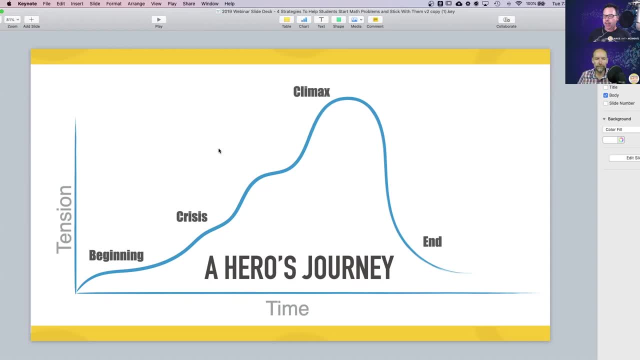 And finding Nemo. And finding Nemo has the hero's journey model as well. Think of the father. Oh, I even forgot the father's name. The father has to Marlin, Is it Marlin? I know Dory is the other right. 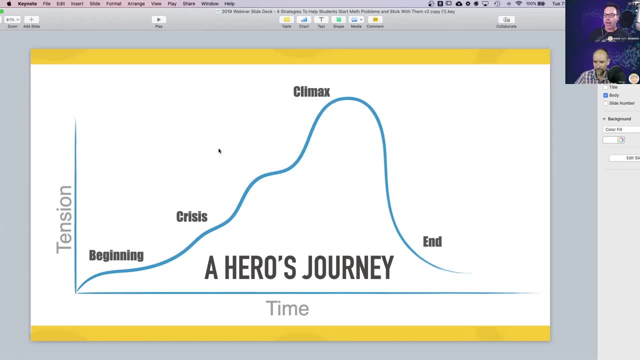 Now Dory is the guide on this story- Kyle So Marlin. he's got to save his son, He's got to find him And he's going through all. Think of all these struggles that he has to swim through. 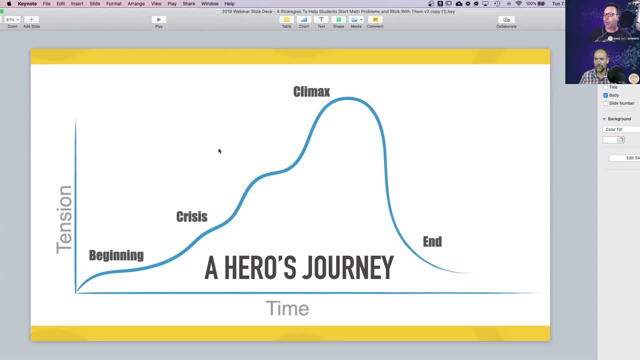 But along that, Dory, even though Dory can't remember anything, Dory is the guide. He's the guide that helps him through that struggle, And so every one of these stories kind of ends the same way: You get to this climax. But the climax wouldn't be worth it if the hero didn't go through all of the crisis. They didn't battle the forces, They didn't learn about themselves. They didn't go through this struggle, Because it's the struggle that really makes that climax worth it in the end. 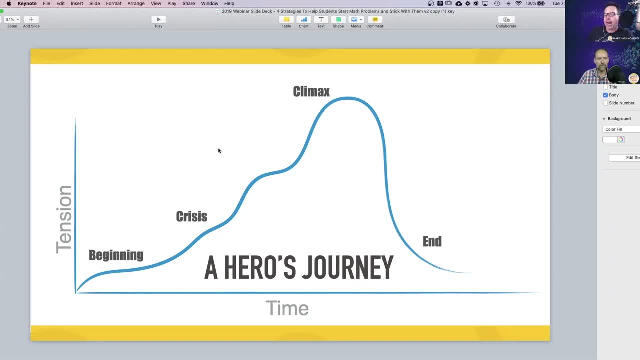 Especially for the viewer, the reader of the story. And what happens at the end of all of these is that the hero will return home, And it's not the same home as before. Things are a little different. The heroes also learned about themselves along the way. 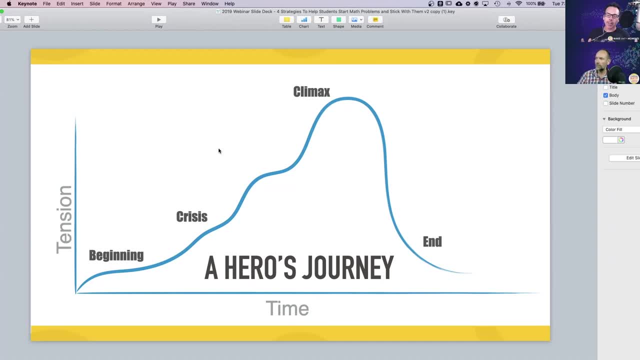 So it's not exactly the same home. Things have changed a little bit. This is the way the hero's journey is described, And it's a cycle, because the hero would then do this again and again, and again, And it happens again and again in so many different stories. 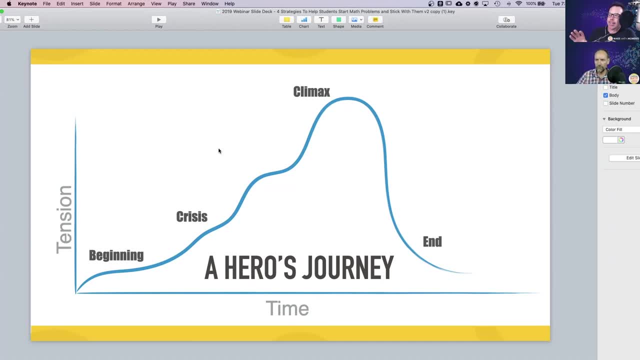 And why we want to outline this is because this technically, Even though this is a storytelling element, we know from, From seeing this curve, you know, you can imagine this curve, this time axis, that the tension rises and then it comes to a peak and then it falls. 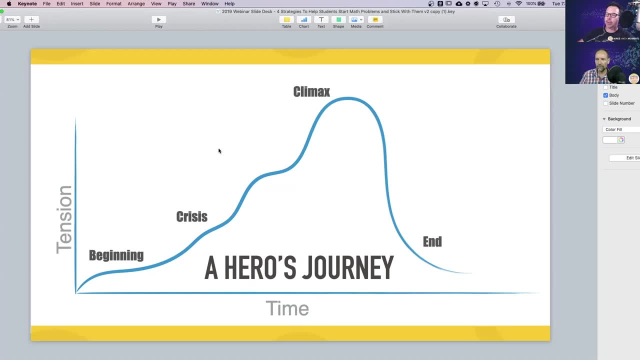 Okay. so if you want to think about this, there's like a skewed graph to the right here where we've got this tension rising up to the right, hits a climax and then falls because he goes home. And what we noticed when we saw this, when we were at that session: 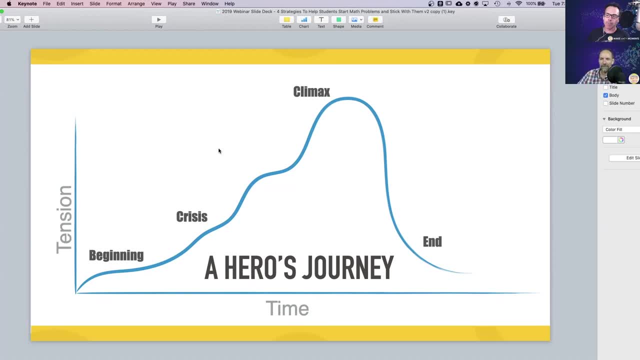 we said that that's not just a hero's journey model of storytelling. This is, This is a learner's journey. This is This process, like this struggle, this kind of graph that we've created here, this skewed model to the right where it hits a climax, is like every time we learn something of value. 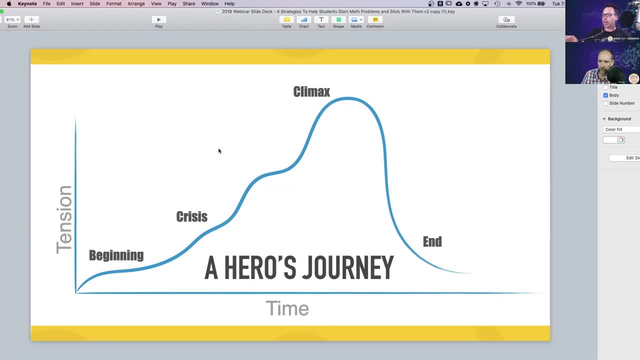 we go through this model Like- think about Kyle. like you play the guitar, You know you had to learn how to play that guitar. Like in the beginning it was. You were set on a path You knew you had to like. 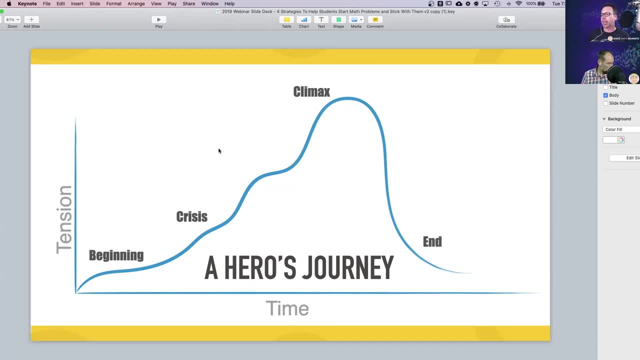 You wanted to go somewhere. And then think of the battling, the forces of Like, think about your fingers, Think about the chords, Think about like all of that work that you had to put in, Like it wouldn't make you knowing how to play the guitar now as worth it to you. 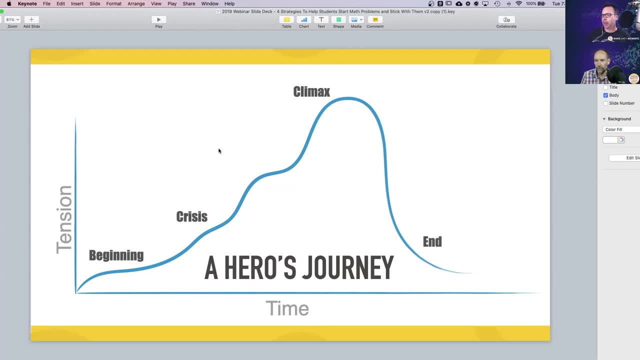 unless you went through all of that struggle and hardship right Like it was. It's that part that defines that moment where it's like this was worth every moment And, if you think about anything, you've learned something that you really and truly value. 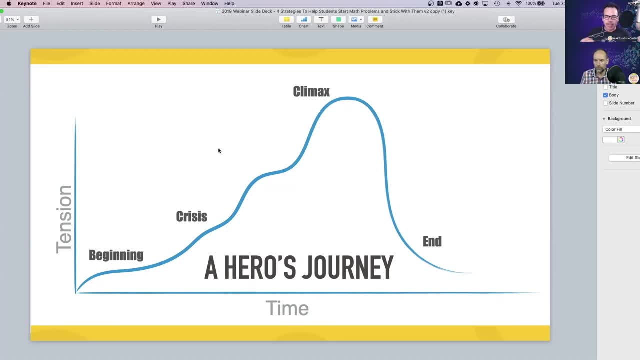 You do go through that model where you have to, Like you have to. It's that struggle that you attach value to that learning And that's what we want to happen in our math class And when we think back, Kyle, to our gradual release of responsibility. model of math class. 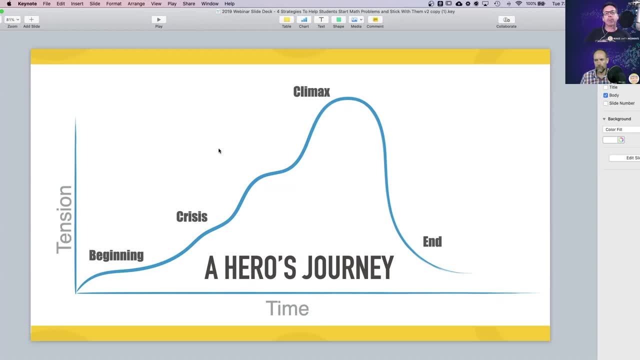 we weren't allowing our students to go through that struggle. We were just saying: hey, I'm going to help you out here, I'm going to show you all the steps, I'm going to give you all the examples so that you don't actually struggle. 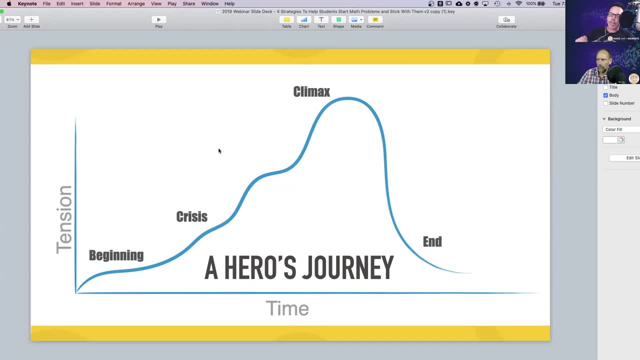 because I wanted to make math easier. And what we were doing? By taking away that struggle, we were robbing our students of that productive struggle, attachment of value to that learning. And this is why kids say like, why do I have to learn this? 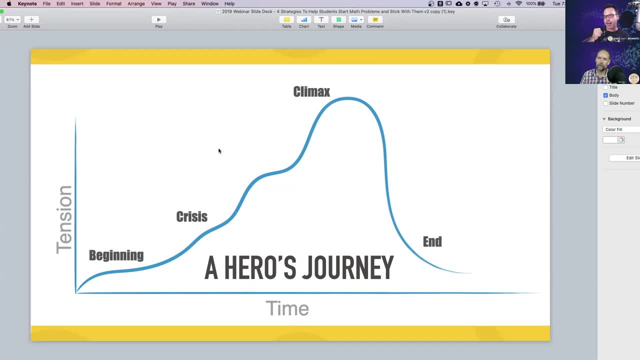 They don't care anymore. It's because we've taken away that like battling the forces of evil part And there's no like need to want to learn this, because we didn't have attached any value to that learning And that's been our mission, right, Kyle? 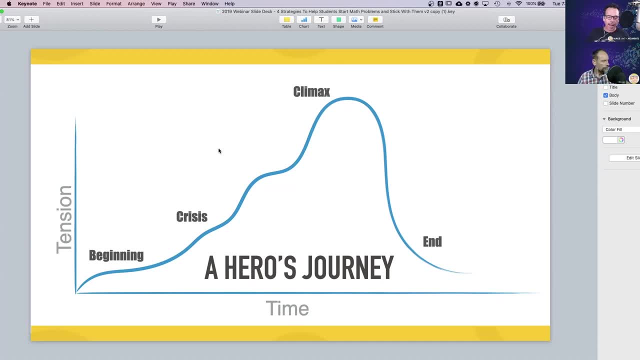 Since day one of us- Since day one of us doing this podcast or our courses or even working with our students- is: how can we craft this hero's journey model in our math classes, rather than kind of just doing what we used to do with this gradual release of responsibility? 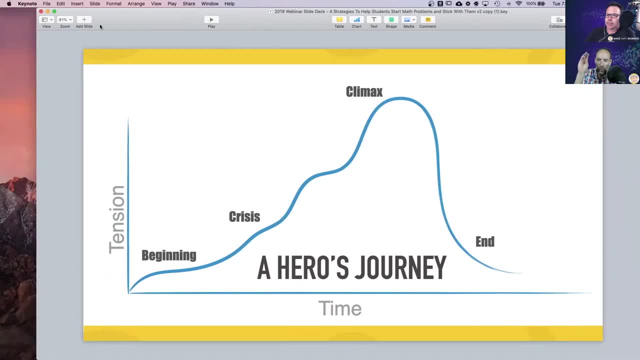 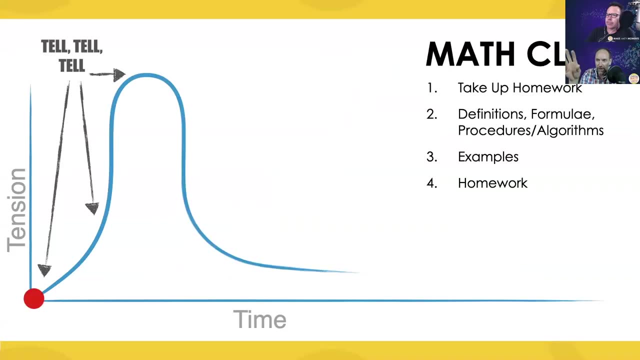 Well, it's interesting too, John, because when we go back to when we were both in the same room, sitting next to each other watching this writer from Pixar sort of take us on this Idea of the hero's journey, And I think we knew it in the background, you know. 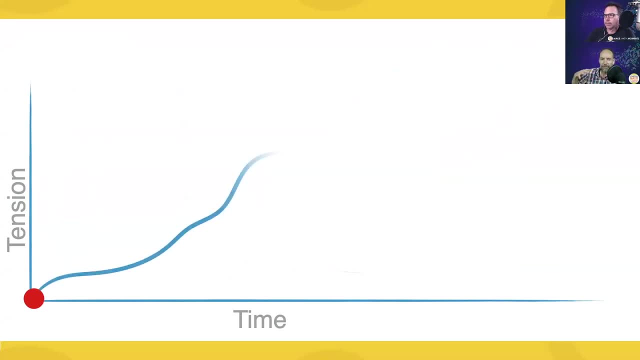 like we sort of knew that this sort of existed, but it was like because we were there through the lens of math teachers. it immediately sort of like had this effect on us And we started to realize what we were trying to do. Because even back then, John, I don't know if you remember this- 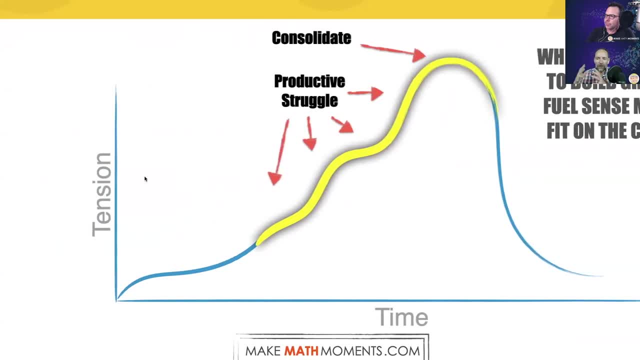 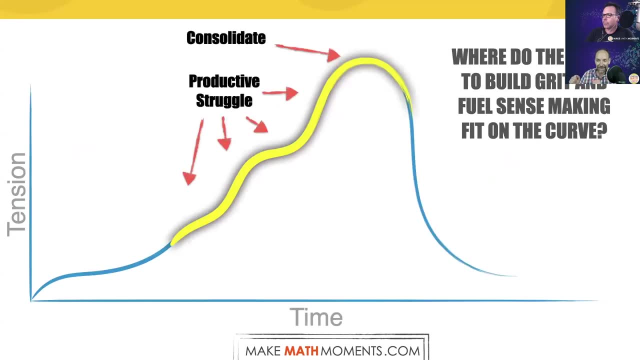 but at that time we hadn't crafted our three-part framework, Like we hadn't put that together. We were experimenting With three-part or three-act math tasks And if you think about the work that Dan Meyer has done and his blog post, which will link up, you know 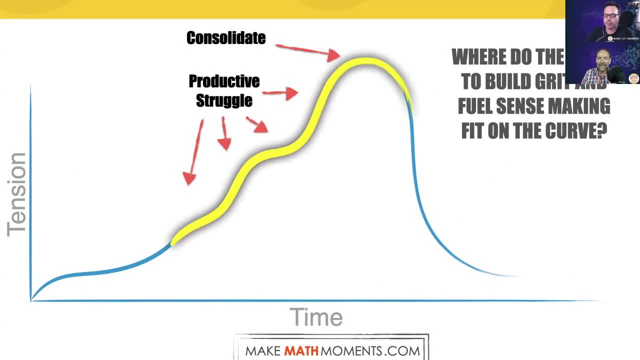 the three acts of a mathematical story, although he talks not about the hero's journey itself. he's talking about three acts. The three-act model is much or very similar to the hero's journey, Like a lot of those same elements are there. 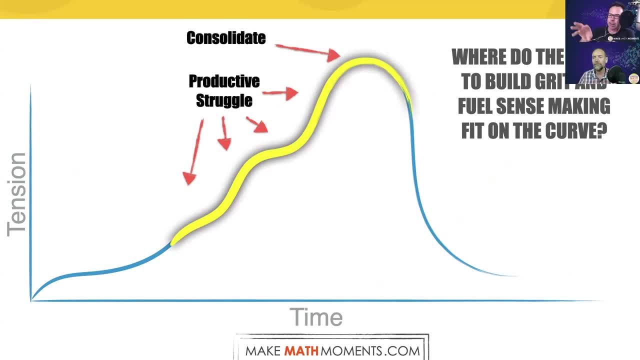 For sure, The three acts are there right. You've got the beginning. the middle, The three-act part is the struggle right, The attaching value to that learning, And then the end is when Dan would say: you know. 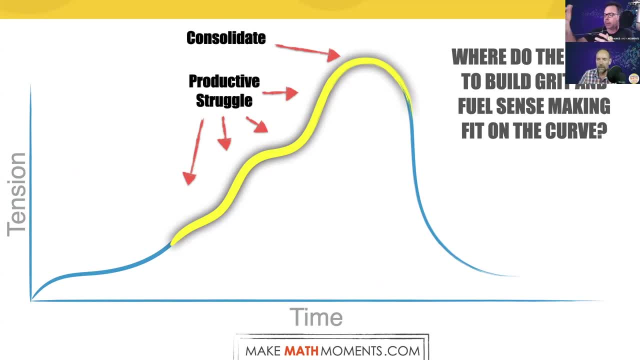 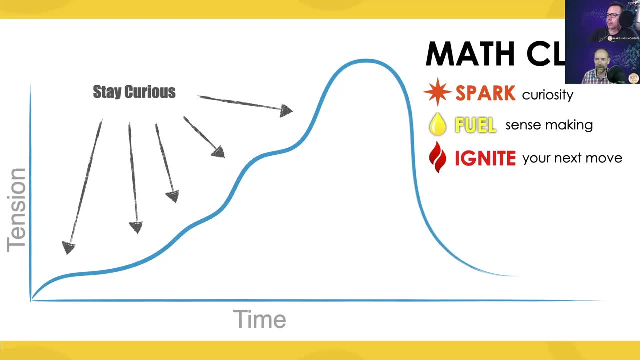 we've got to reveal the answer here. That's like, hey, that's the climax, Now we're going to head home, Yeah, And these are things that, like you know, started to kind of align, Like the stars started to align for us. 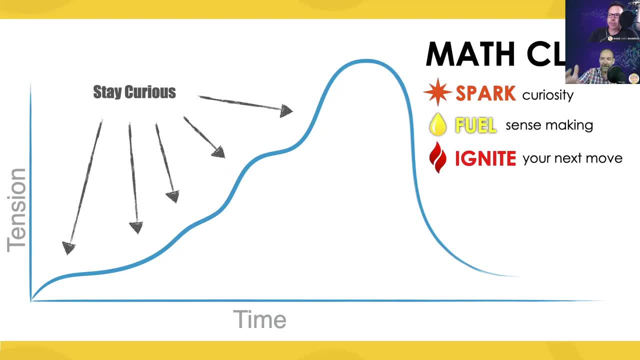 And you know we started thinking about, like, what does this actually mean? So, as you can see on the screen for those who are on YouTube, you can sort of see this curve, our old curve, which was sort of like this: hey, I'm just going to tell you. 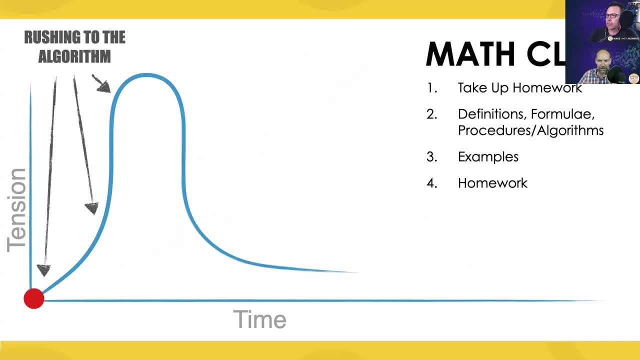 you might, you know, struggle for a moment, but you know, with enough practice you'll get over that hump. And it was that rush to the algorithm When we flatten this curve out- and I say flatten, but more or less have a gradual increase of this curve. 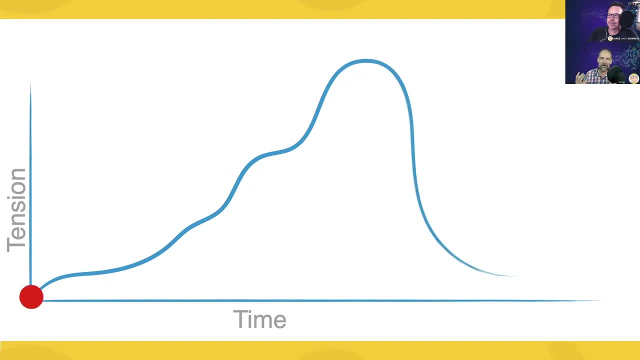 you start to see these elements that we're talking about Like. you start to see curiosity and we're trying to keep kids curious as long as possible. And how do we do that? Well, we do that through the curiosity path, right, So we provide opportunities to notice and wonder. 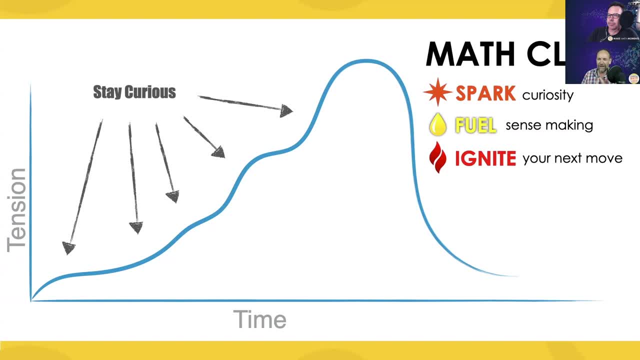 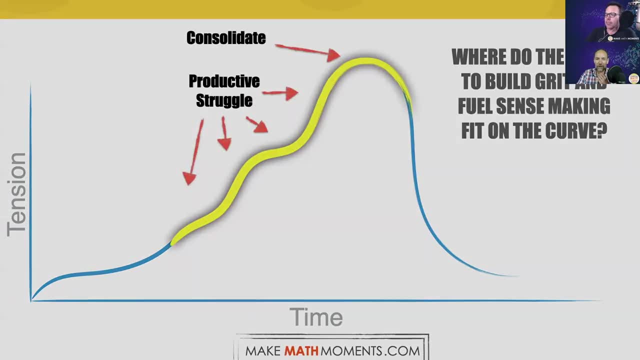 for students to kind of anticipate, you know, by withholding information, and then we get them estimating. And actually, John, something I'm going to share because I actually was Googling for this image, thinking it might come up when I share my screen: 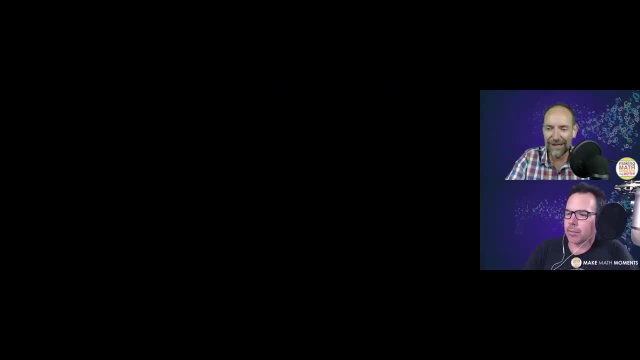 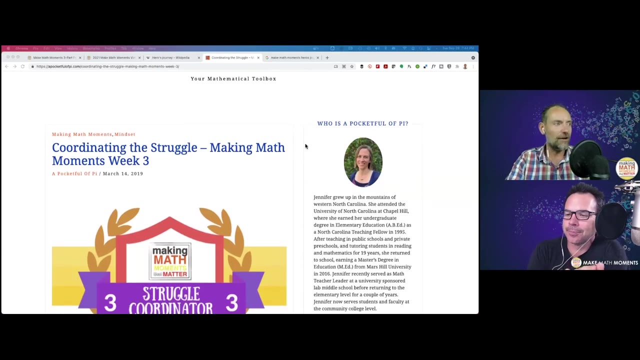 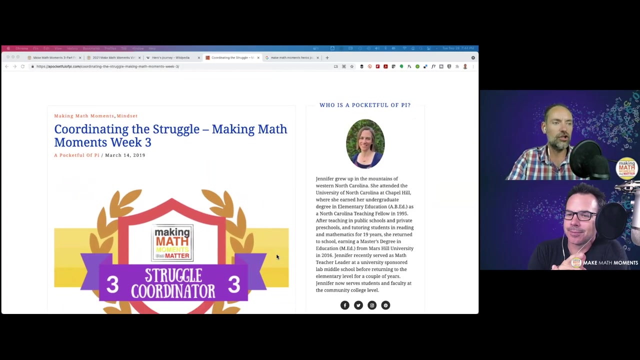 What's really cool is that what came up on Google when I looked was actually a former, a former workshop participant who had reflected on this very lesson, And I'm not going to say the last name. I know the last name, But I noticed on her website she doesn't have her last name anywhere. 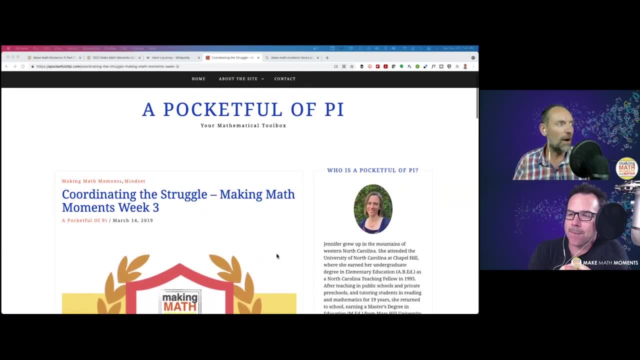 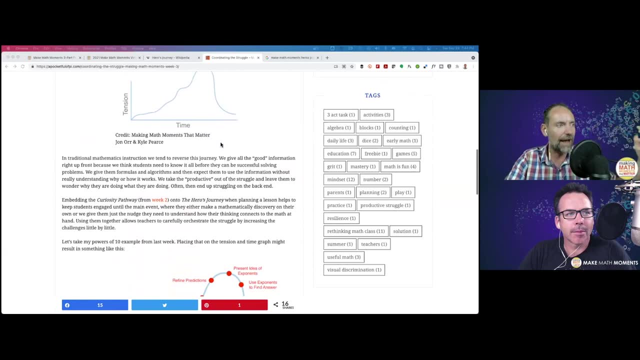 So I'm going to respect that. So it's Jennifer. The website is apocketfullofpiecom. And down here, what's really cool, she kind of goes through. you know the impact that lesson had, But then she also made her own. 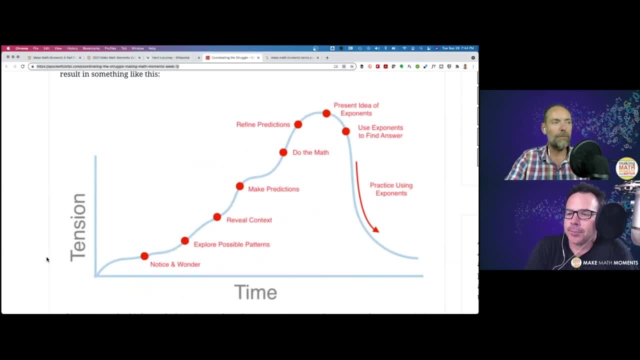 She took that curve and she actually like walked us through based on her lesson for exponents. So she talks about, like the notice and wonder: let kids explore possible patterns, reveal the context, make predictions, doing the math, refining predictions- And then you see like she kind of goes over the edge of this curve. 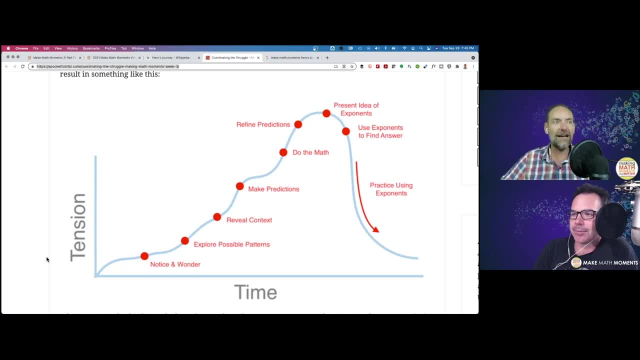 where now we start, like we consolidate this idea of exponents. Maybe it's exponent laws they're looking at. whatever it might be, all the way down to now we can do some of that purposeful practice, as we had mentioned. 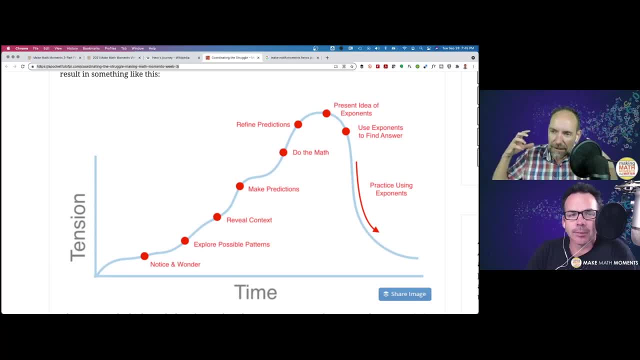 Now that purposeful practice has some, like some, some you know- legs underneath it right, Like it has something going on there where now I can go. I can connect it back to the story, which is our math lesson. 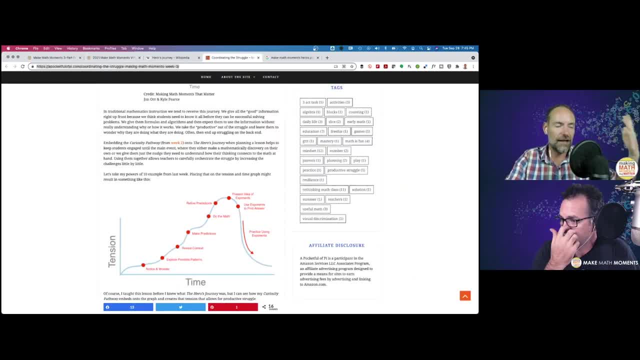 And you know, for me this was great to not only see that a student who went through the online workshop has an awesome reflection online sharing how they're going to try to be the hero instead of the guide. It really like the other way around: they're going to be the guide. 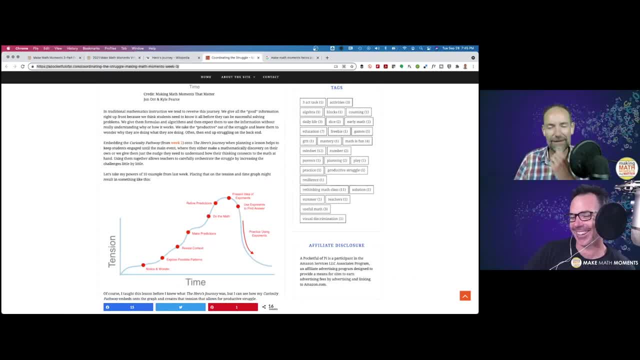 Yeah, sorry, the guide, not the hero. Please don't, don't be the hero We're. I think we've been the hero long enough. Right, we're the guide. When, when we're crafting these lessons, like, if you think about it as a story. 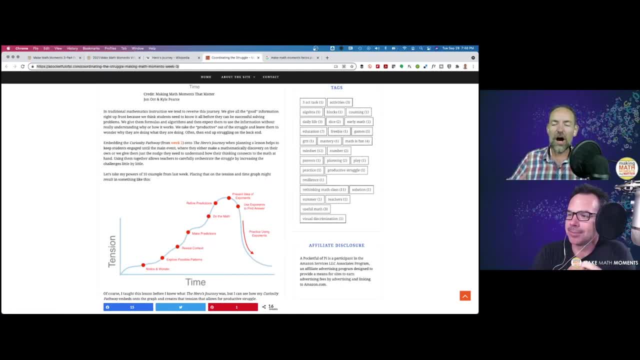 and it doesn't always have to be, you know, like a knock it out of the ballpark kind of story, but it does have to have something there for students to kind of like: join you on this journey, right, And you want to guide them through this journey. 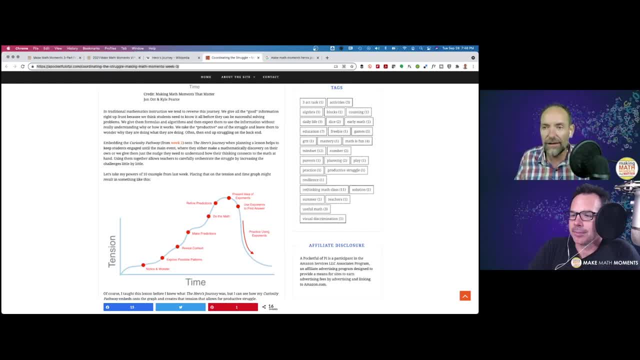 And they have to obviously want to be a part of that journey. They don't want to just follow and mimic, which is what John and I have done for so long. So like hopefully thinking about your math class as a lesson, as a story that students can think on. 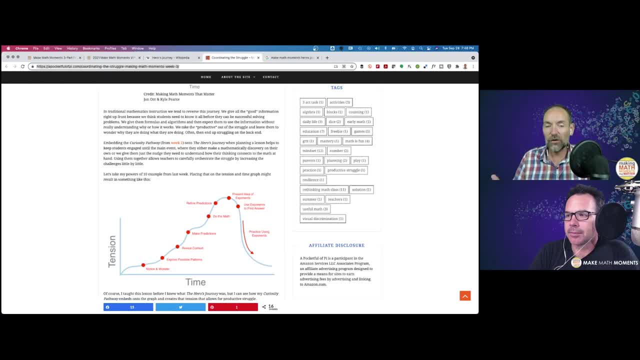 you know, and, and the example that I have in mind, my most recent- I was in a classroom today in person for the first time in a long time, which was awesome, But we were in person and the whole story of the context- 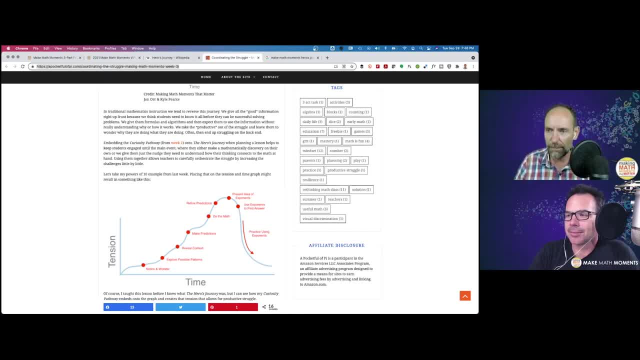 we were multiplying fractions and we used the shoveling, the driveway problem And to be able to have this conversation and everything throughout this lesson was sort of like connected to this context Right, Where students were all on the same page, being able to reference the same driveway and being able to use fractional language. 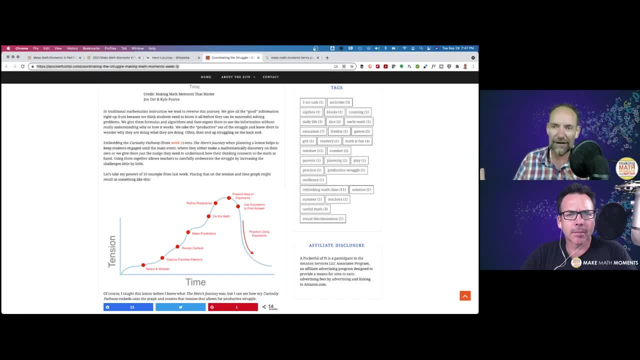 Like I haven't heard students use quite often because it's so disconnected It really does like very quickly you start to see that, wow, I could probably reference this particular context weeks from now And students will like be able to come back to this moment. 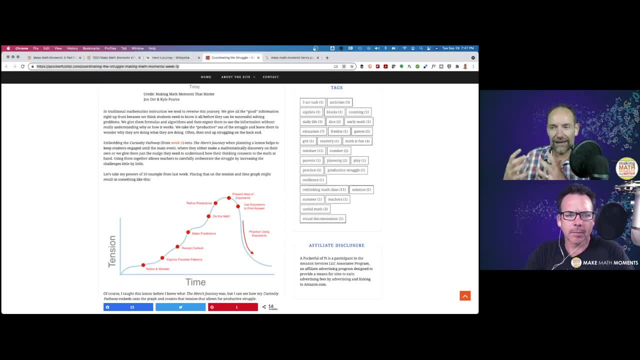 and relive at least a portion of that lesson and that learning that we were hoping that they would learn, That we were hoping that they would elicit from the experience. Nice, nice, Yeah, that's another great example of that. And going back to what you've got to hear on the screen about that student of ours, 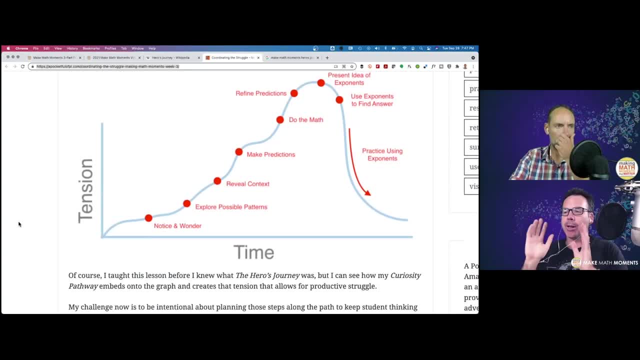 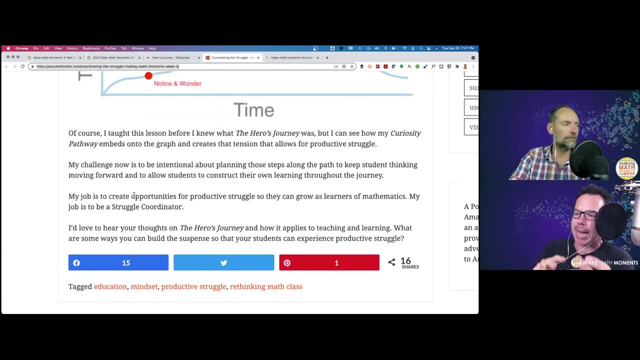 from the online workshop. that is actually like they've done a great job, because that's actually one of our lessons in that workshop is to take the hero's journey model and map your lesson on top of that diagram. So super exciting to see that. 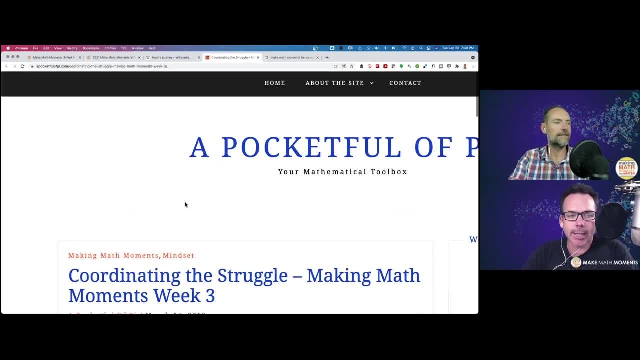 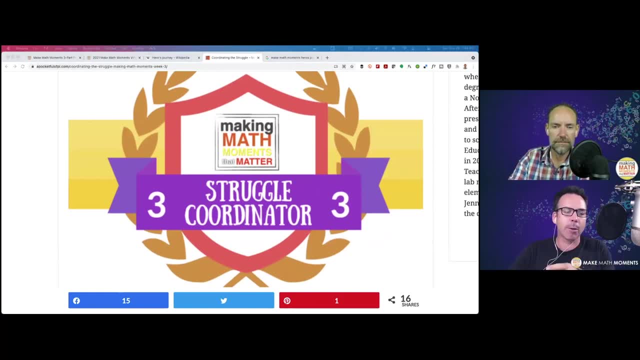 We're going to put that blog post in the show notes- a link to that. I was typing that just a moment ago, so on the fly here, So super excited to share that with you Also. another thing that we want to share with you is more resources on storytelling. 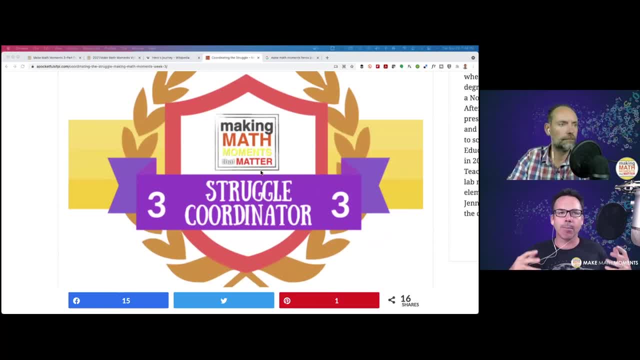 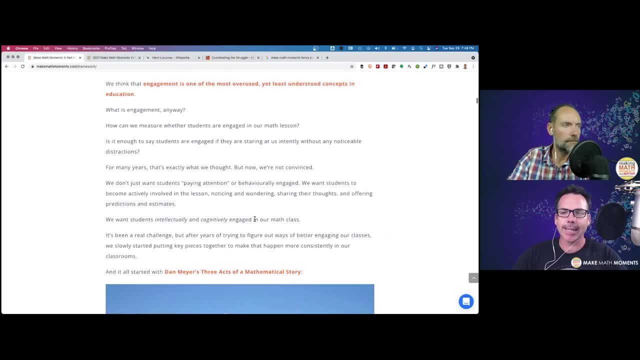 And I think the storytelling aspect can be, you know, done so many different ways, Like so much of what we, you know, what we can do in our math class, is tied to storytelling. Like, think about this, Think about assessment for a moment. 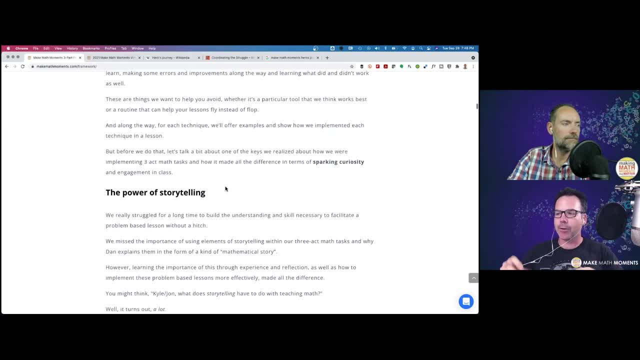 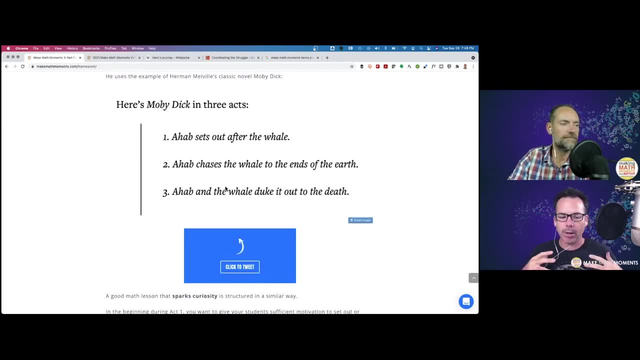 Like assessment is like you're telling the story of their student's journey through assessment. Like: how can we do that with you? know the tools that we have at our disposal. Like: how can you share that journey with your students? 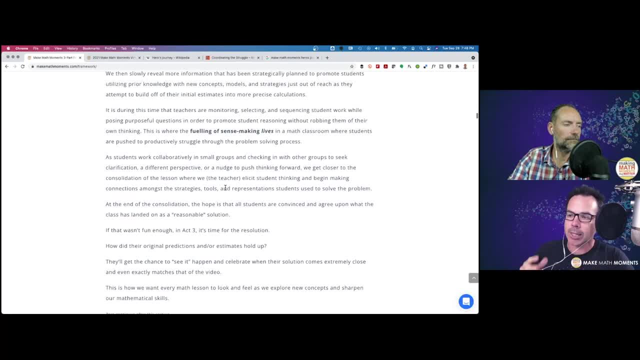 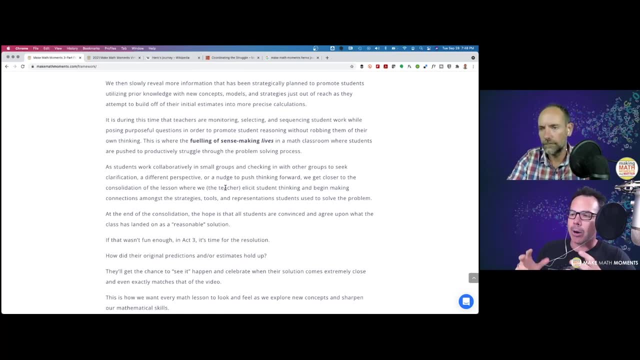 Like: what are you doing for assessment? Like, if you can think of it more as a story, then I think that will actually change some of your mindset around how you view, say, evaluations and tests and assignments And the way you're assessing. 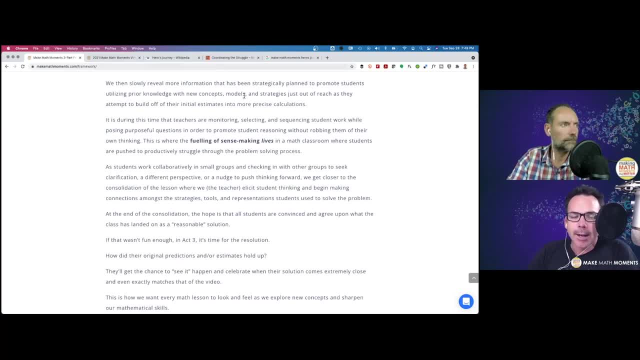 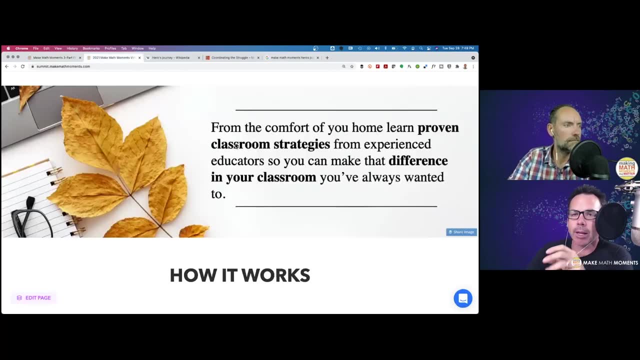 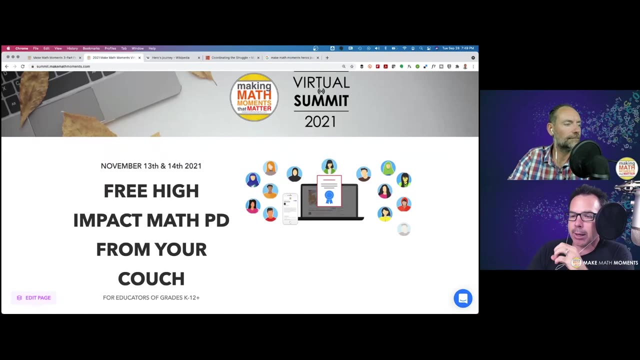 Because it has helped me do that significantly, Kyle. another resource I want to share here is we've got the Make Math Moments virtual summit, the 2020 virtual summit, coming up at the time of this air date- It's in November, And November 13th and 14th is coming up soon. if you're listening to this episode when it goes live. 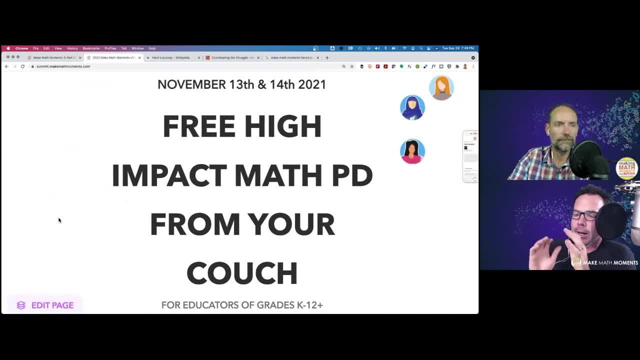 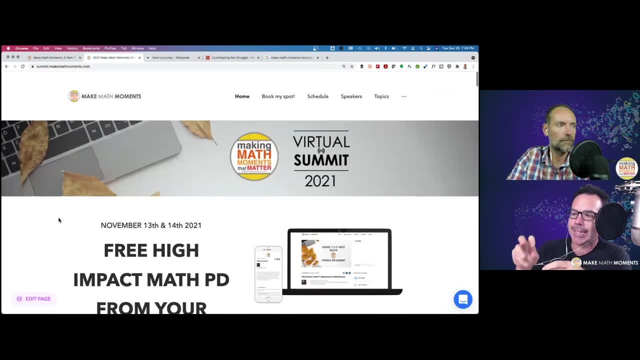 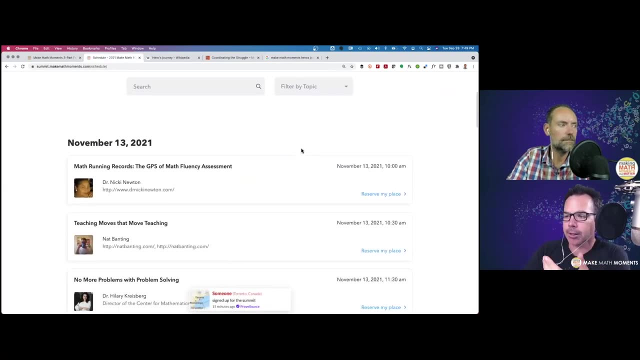 or in those weeks of November 13th and 14th of 2020.. And I really want to point out, because there are some sessions in this summit completely dedicated to storytelling. The first one is from Sunil Singh Kyle. can you maybe describe what Sunil's session is about? 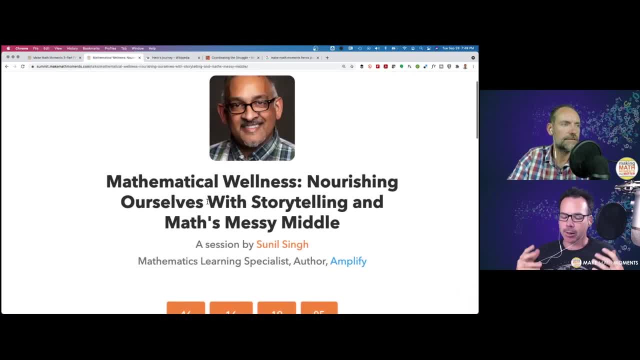 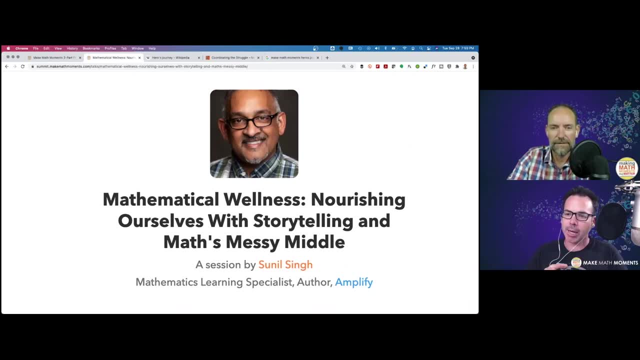 Kind of like his kind of synopsis here, Because I'm really excited to see this session And also he's got a book coming out all about storytelling And mathematical wellness. Super exciting stuff from Sunil lately, Yeah, And Sunil is awesome. 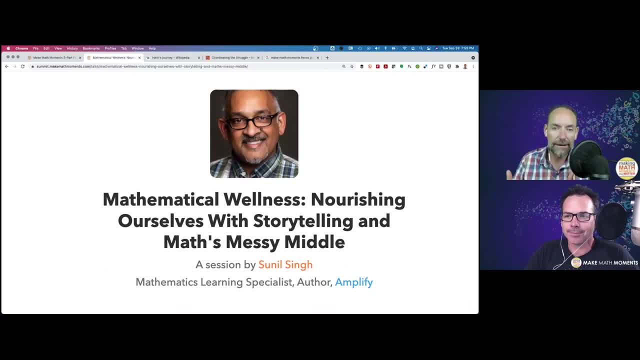 I am proud to be able to call him not only a colleague but a friend. You know he has been someone that we have had the pleasure of learning with and from. for the last, I would say what? Now it's got to be six, seven, maybe eight years now, going all the way back to some of our earlier OAMEs. 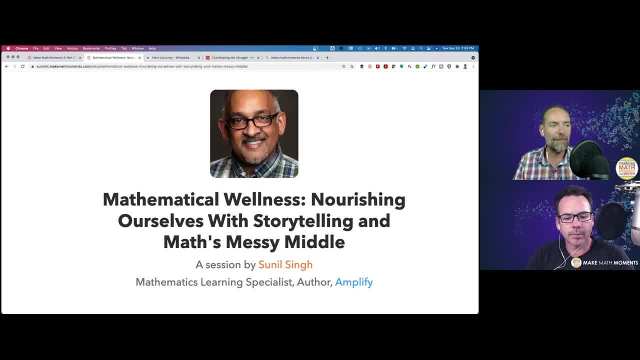 But Sunil is going to be talking about mathematical wellness, Nourishing ourselves with storytelling. There's that storytelling theme and math's messy middle And basically like what Sunil he's talking about, and his descriptor goes something like this: He says: one of the most negligent things we've done in mathematics is that its purposes have always been directed externally, to supporting and providing for society. 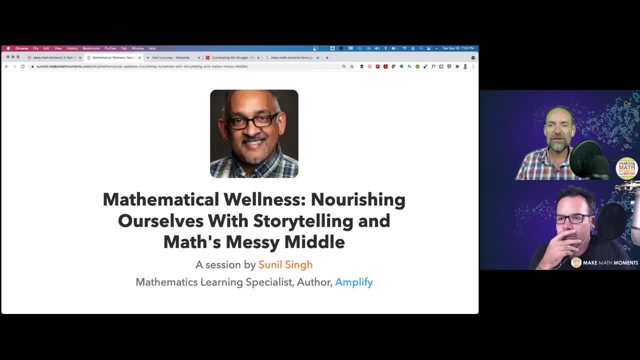 The focus has also taken a toll on our students And teachers, who must engage with mathematics through a lens of compliance, performance and competition. How true that really is, And that rings true there. Our energies have been consumed by this, in this toxic landscape. 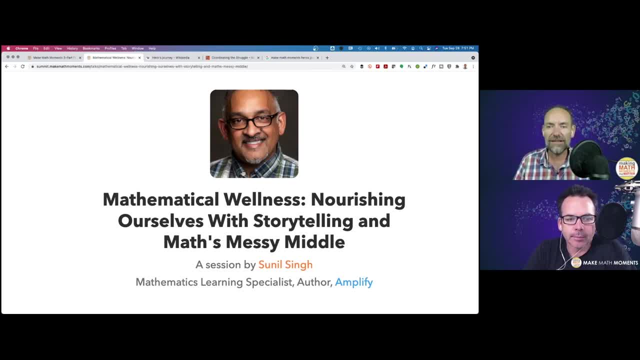 But our failure has been that we have neglected ourselves. What purpose does mathematics have with our life's journey? To answer that question, we must approach math in a completely new way. We must embrace confusion And uncertainty. So there's that productive struggle message, kind of coming out with excitement and not trepidation. 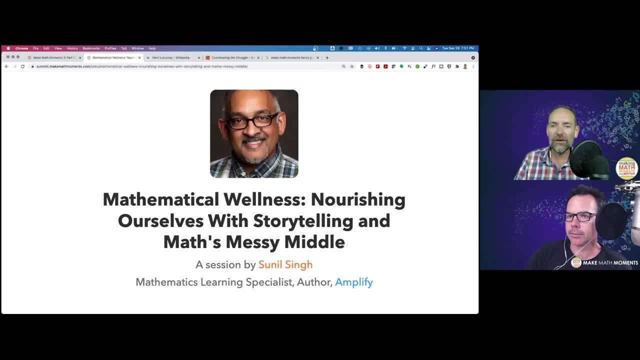 We must do this because it's been the entire historical narrative of the history of mathematics. We must reclaim its human power and purpose. Wow, Like talk about. you know that is impactful, And I know that Sunil has spoken on some of these concepts in the past. 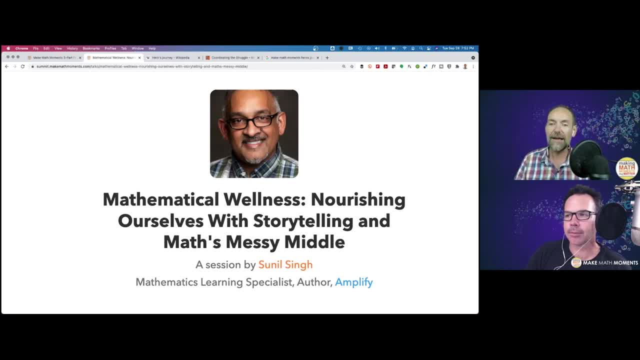 And he's been a part of them, And he's been a part of our previous summits And we've also had the opportunity to support him whenever we're at NCTM and OAME. We always like to go and hear what Sunil has cooking. 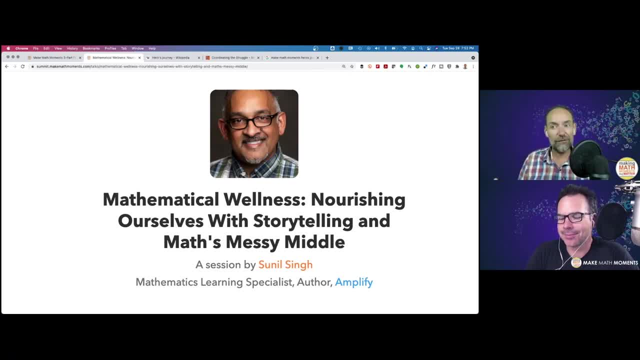 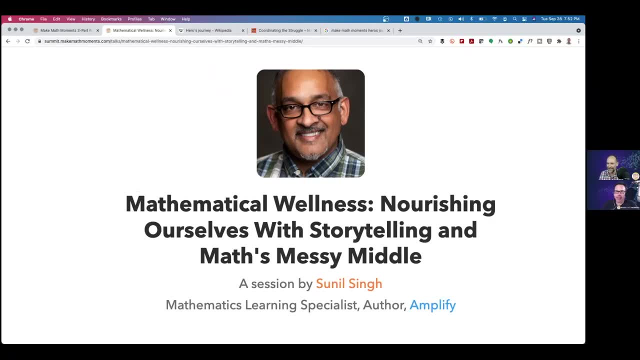 And Sunil. some people might not know this, unless you've gone all the way back to one of our first episodes. really, I think it was what- Episode 5 or 6 or something like that. I think he's like 12 or 13.. 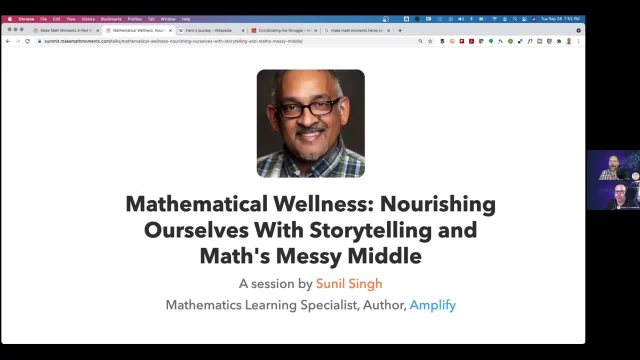 Okay, One of our first episodes. So he's way back there And Sunil actually was a high school teacher and actually walked away from the profession, you know, because of some of these things that he's discussing in this description. So Sunil is going to be talking about the why, like why we need to do these things. 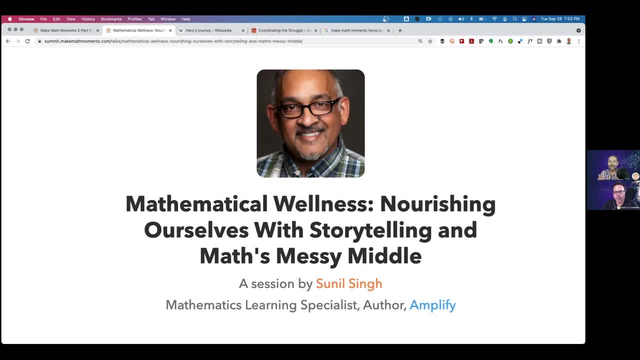 But he's also going to give you some ideas on what that might look like and sound like, And I'm sure you know, by the time the summit comes out we'll be close to him releasing his new book Chasing Rabbits. 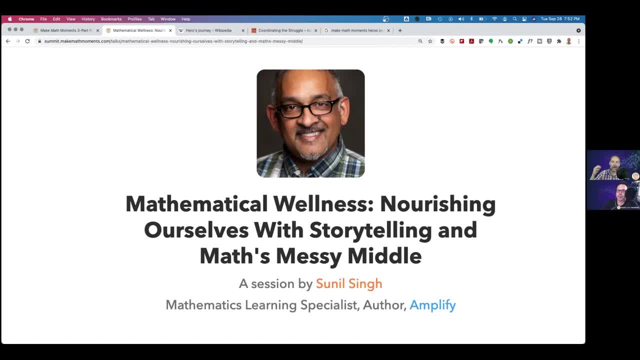 So that will definitely be another support as well. So I think your first step when it comes to getting the storytelling piece here and trying to figure out, like you know, mathematical wellness, check out Sunil's session at our virtual summit coming up. 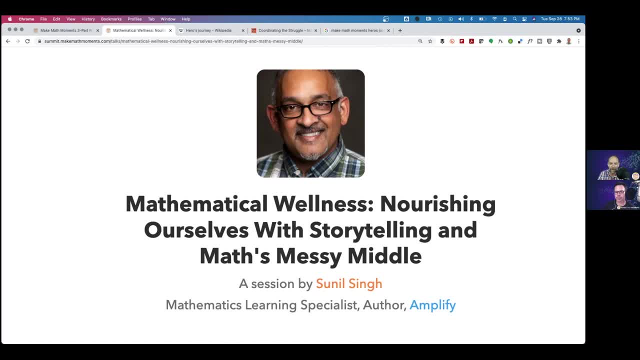 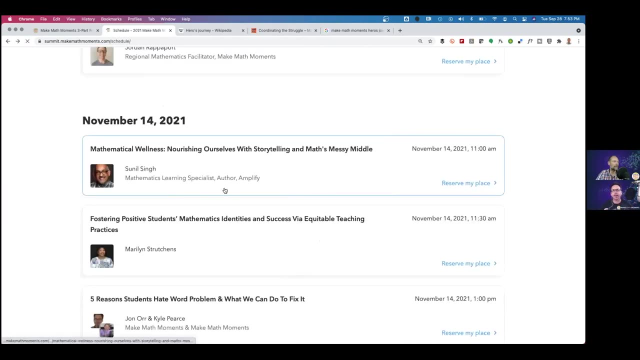 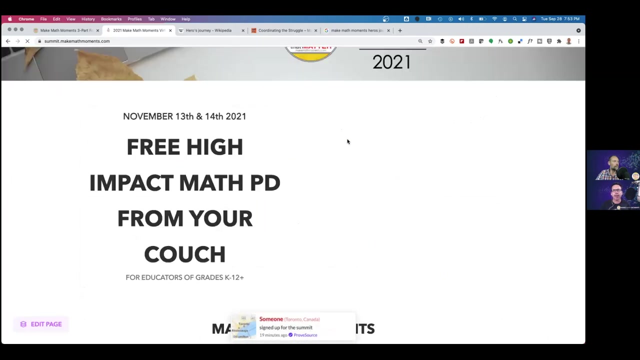 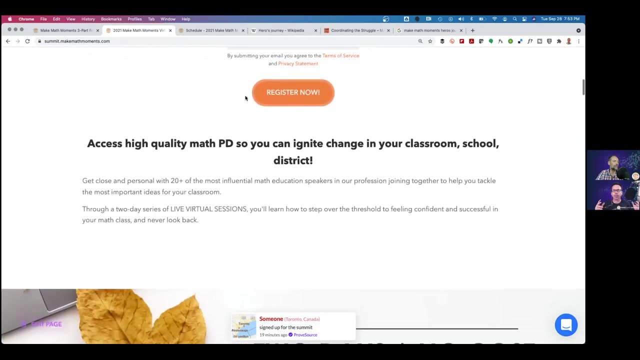 That's makemathmomentscom forward slash summit. if you haven't registered yet, Yeah, for sure, And don't forget, it is completely free. Kyle and I, you know one of our main missions- Yeah, With what we do here on the podcast and the summit and our webinars that we hold quarterly every year- you know, four times a year, or I guess three times a year, Kyle- is that our big mission, our big why is that? we want to provide as much professional development to as many educators. 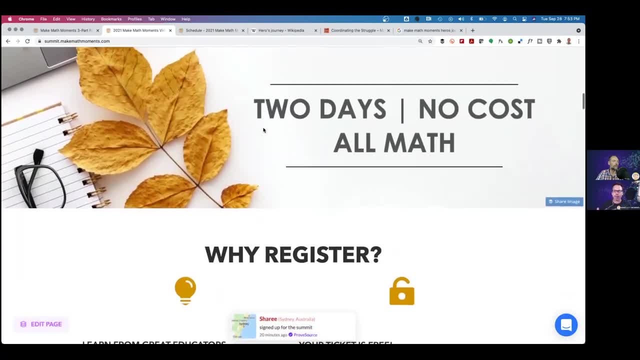 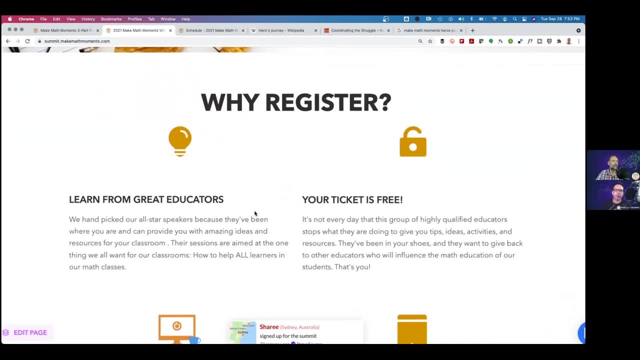 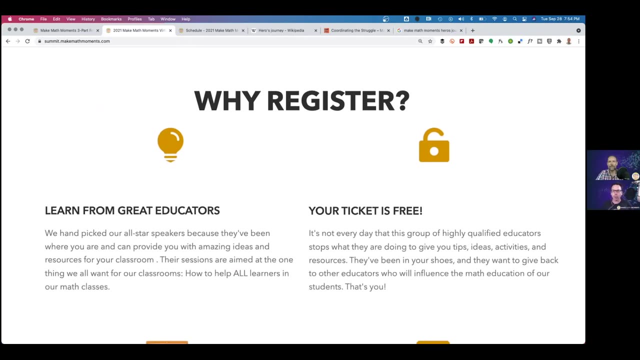 We want to make it accessible for as many people as possible, And this part of the reason is why we do this podcast is podcasts are completely free to listen to. We want to provide you that professional development this way. but here's another way that kind of digs a little bit deeper is to get in sessions with folks. so all of these folks know that this is a completely free conference and they are still here. 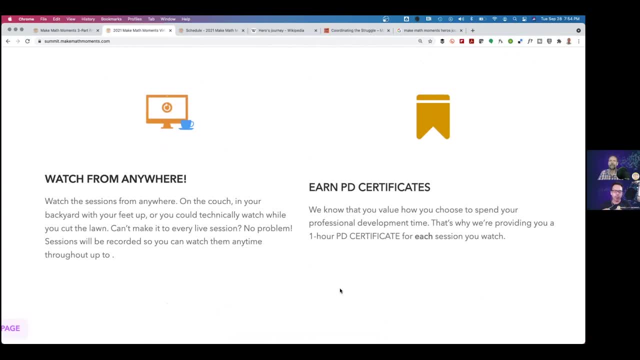 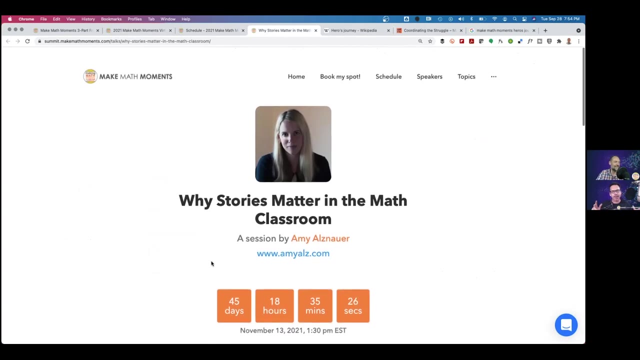 You know helping you guys out, so super excited to bring that to you and as many teachers as we can. Kyle. I want to point out another session here in this year's summit On storytelling And- and this one is by Amy else now, or her title is why stories matter in the math class. so it's like right, right there. 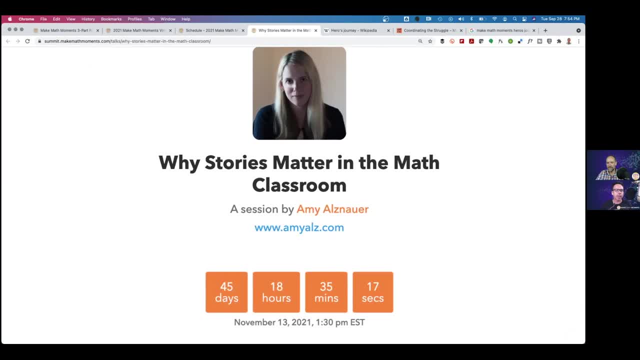 Her description is: stories are the heart of being human, so they belong wherever human beings gather, But especially in the classroom. stories inspire, expand our horizons, they make them kinder and more beautiful. They initiate new projects and offer a common language to help build community. 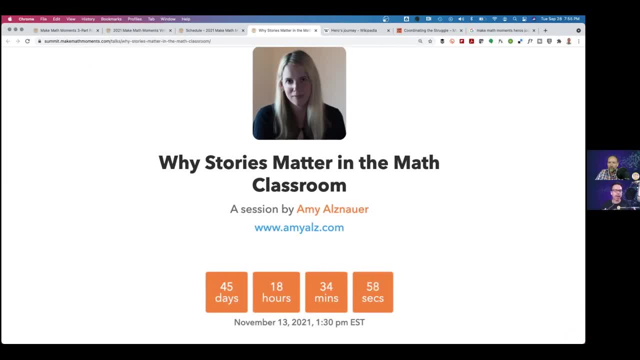 Amy And she's a university math teacher. it will talk about how math stories changed her life and then use her book the boy who dreamed of infinity to show how adventure, learning and community might grow from a single story. so excited to have Amy join us- this is our first. 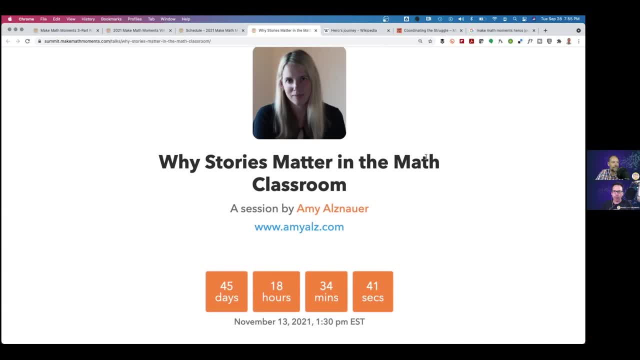 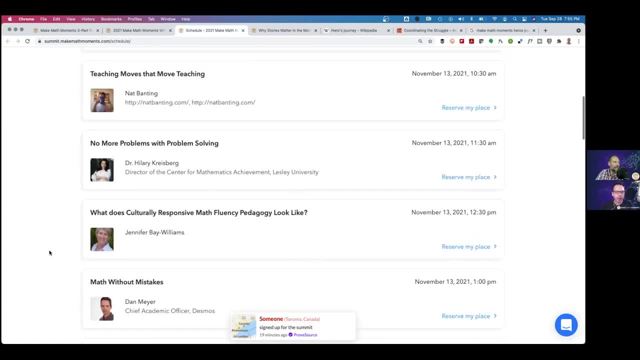 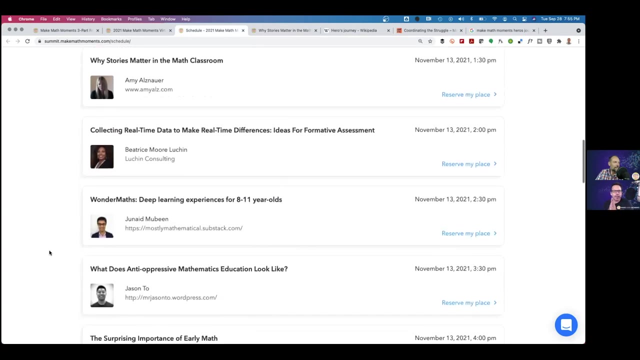 time at our virtual summit and super excited for her to join us and talk about storytelling. we met with her a few times to talk about these ideas and really excited to have her as part of this year's summit already. Okay, We're going to start wrapping up here because I know that we're getting to the end, but but can you let everyone know where to go if they have not yet registered? 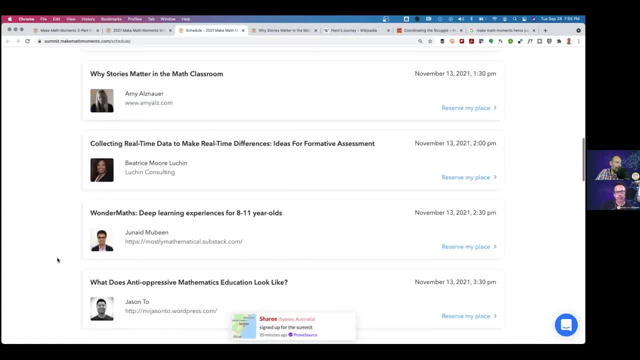 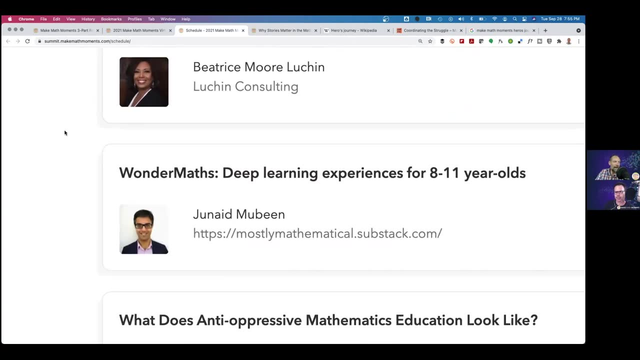 Yeah, absolutely, And I know we did mention that. Dan Meyer and three act math. he's going to be a part of the conference. we've got all kinds of amazing names joining us for the virtual summit this year and you're going to notice like now, that we're talking. 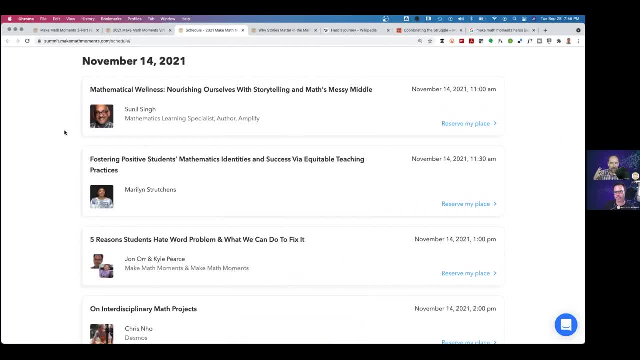 about story. When you watch these presenters, I want you to listen. I want you to listen and I want you to see how they present, and you're going to notice some of the most impactful presenters that we find often use story in order to present their sessions. so you know, story is everywhere. so how can we build this into our math? 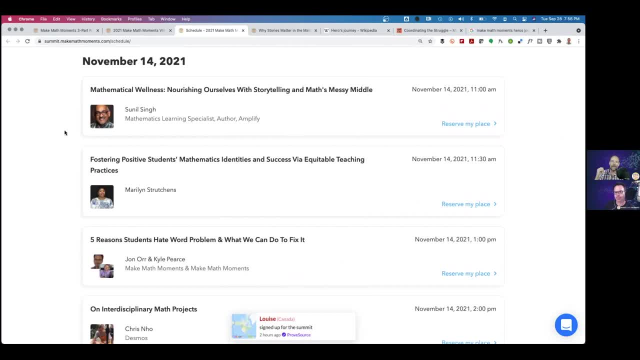 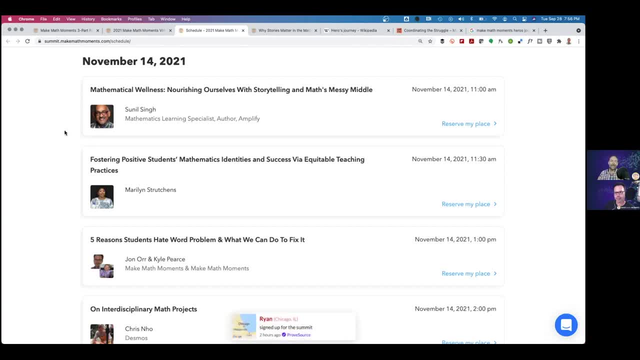 And once you're there- or just Google virtual summit, make math moments. And once you're there, or just Google virtual summit, make math moments- It'll pop up: get yourself registered. we- this is our third annual virtual summit, so maybe you're hearing this. after November, you know, maybe it's it's past the virtual will head to the same link. we're going to have an option for you to sign up so that you're notified the next virtual summit, so that you get a email and you're you know you're- alerted. we usually have over 15,000 participants over the weekend and we're hoping that this year is going to be one of our biggest events. 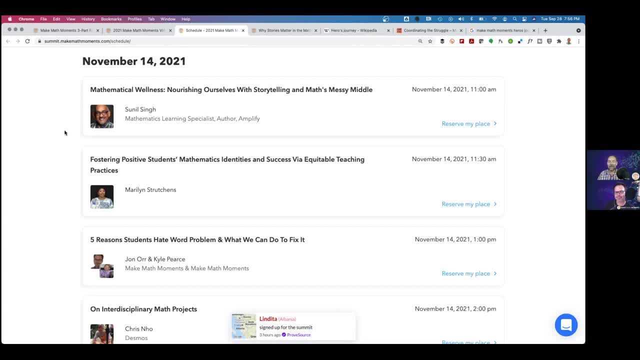 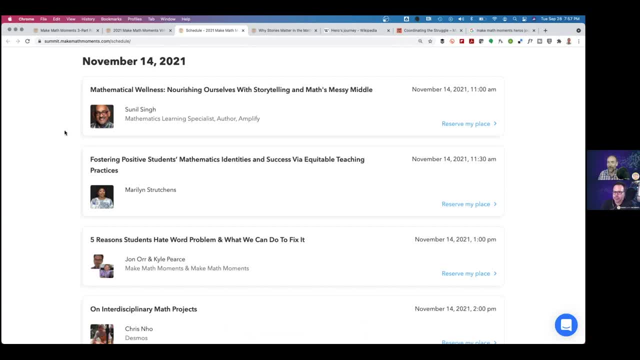 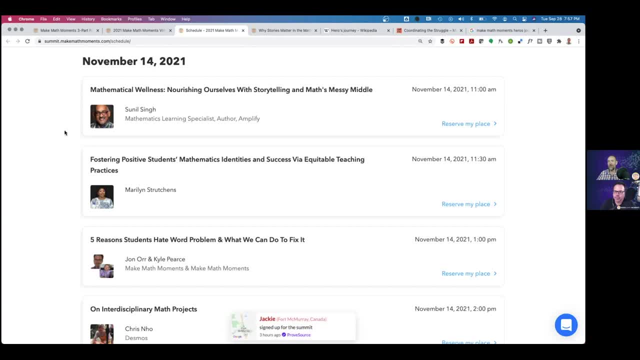 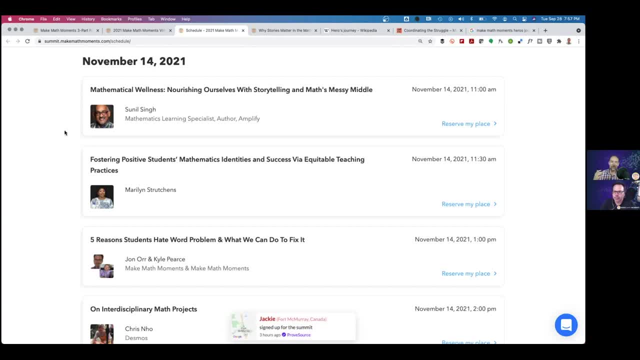 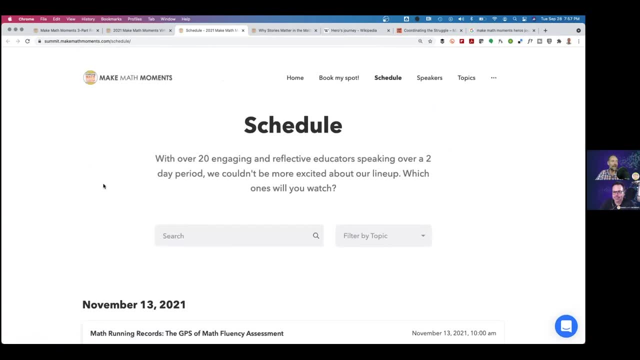 And once you're there, or just Google virtual summit, make math moments. learn how to do that into your in your classroom. make sure to check out our session, as well as many of the other awesome sessions. there's going to be over 25 speakers and, uh, it's going to be. 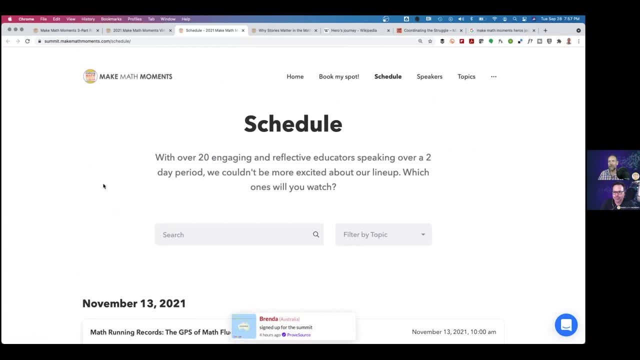 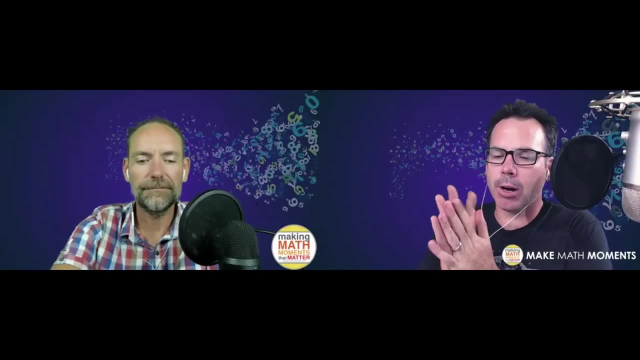 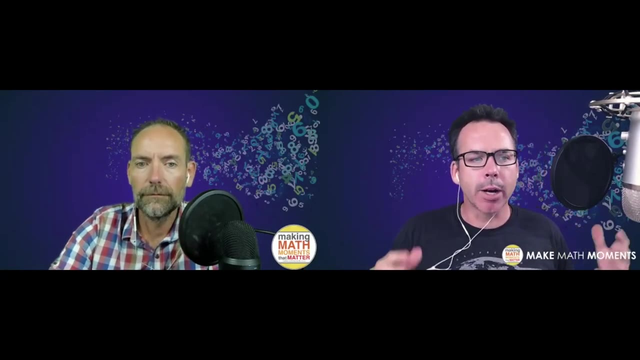 jam-packed. so, uh, i i think we've got an awesome opportunity coming up here on november 13th and 14th 2021. yeah, and just to wrap up here on this particular episode, just to leave you with some big ideas, uh, that we talked about here in, uh, this episode is we wanted to talk about why, you know. 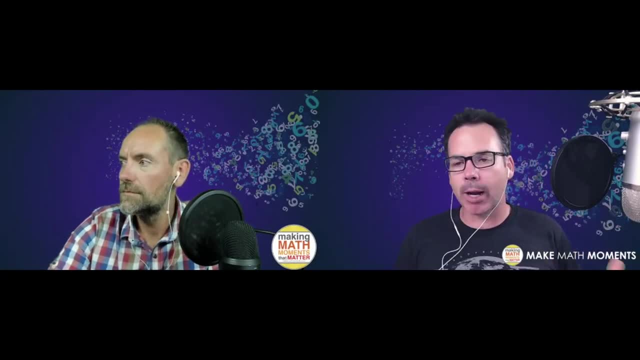 teaching math should be more like story verse teaching, with that gradual release responsibility. really hope uh you're saying, yes, we've done that here, uh, another another thing we wanted to do here was like talk about the necessary elements that will help you craft that story, like how to spark. 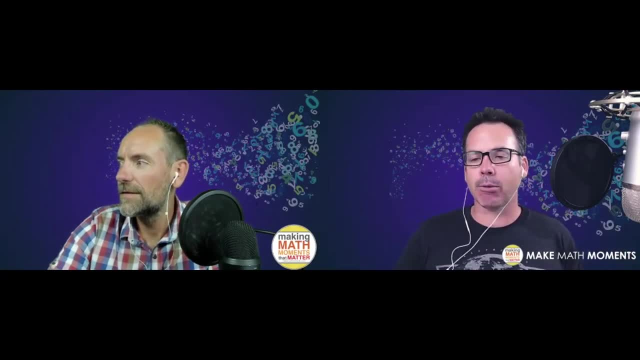 curiosity in your students. it is embedded in our three-part framework, uh, which we've got a link to that in that, that guidebook, in the show notes page here. um, we also wanted to help you shape your lessons so that they can be, you know, addictive in my books, and that's what storytelling can do like how do we get that hook into those? 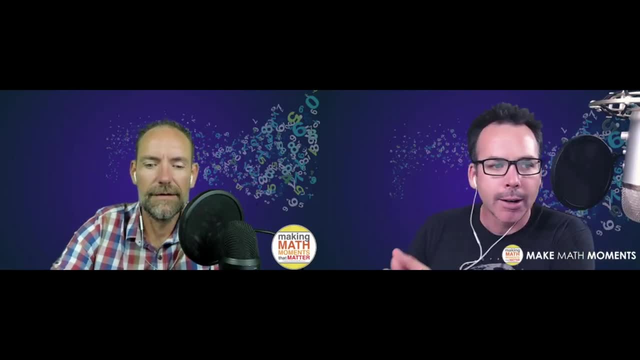 lessons. uh, hopefully we gave you some sparks there and uh, finally, like, where can you go to do learn a little bit more of this? and i hope we gave you some suggestions here in this particular episode, kyle. yes, john, nice job summarizing there, friends. uh, you know if, uh, if you haven't yet, make sure. 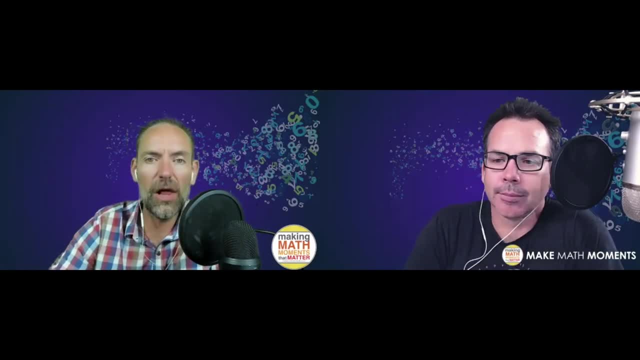 that you do some reflecting. do like jennifer did on her blog. maybe you have a blog, maybe you want to start a blog blog. get out there, do what you need to do to reflect. Maybe it's using your voice memo app in the car and just talking into it to remind yourself of some of the ideas that you want to resonate. 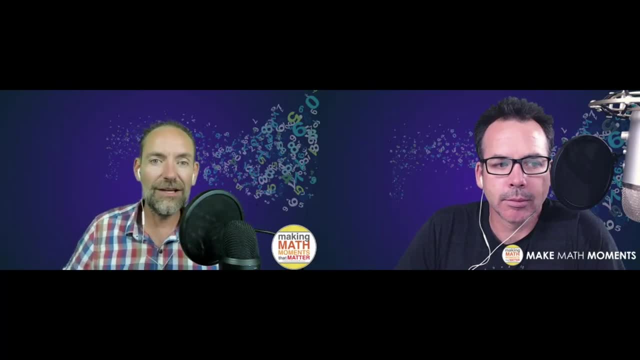 with yourself. Or, like I said to the class I was working with today, I use Peter Lildehall's idea of you know, create a note to your future forgetful self, whatever it is. make sure that you are reflecting so that you know it sticks for you. Hopefully today's message around storytelling. 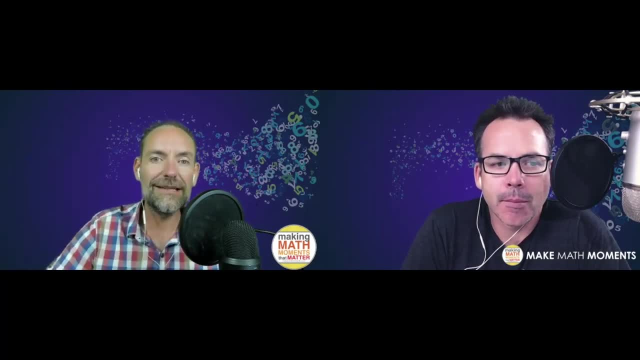 is one that will have an impact and an influence on your lessons, And it helps students learn mathematics in a more effective, sticky sort of way. moving forward, Awesome. In order to ensure you don't miss out on new episodes of this podcast, as we put them out every Monday morning: